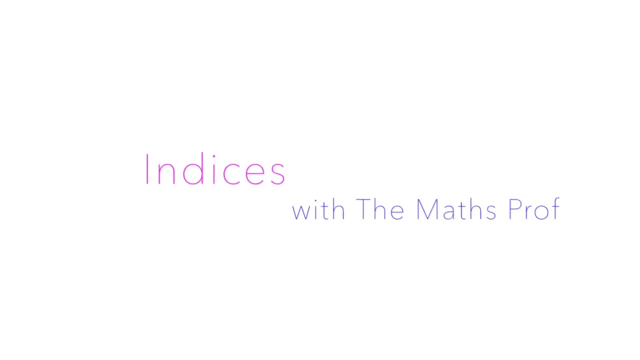 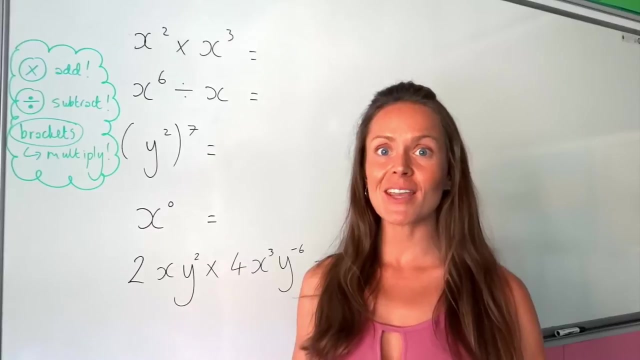 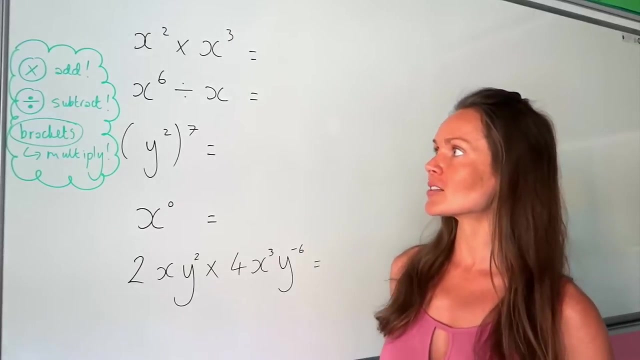 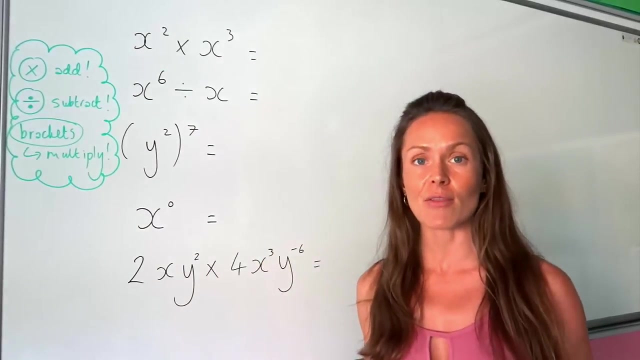 Hey guys, I'm the Maths Prof and today I'm going to show you the rules of indices. So these are just the power rules that you need to remember. So, before I get started, I just want to point these out. These are the basic rules that you need Whenever you're timesing two letters together. 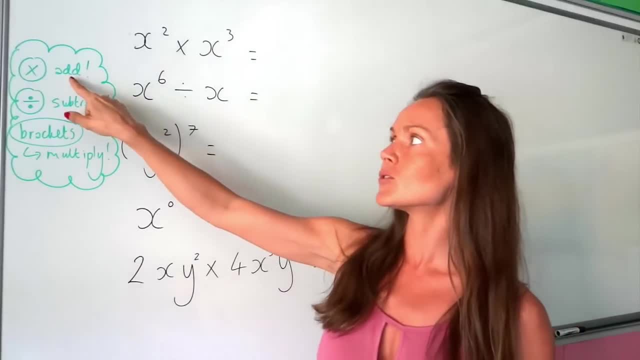 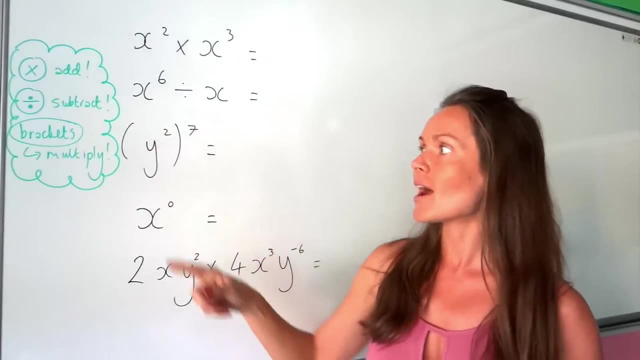 that are the same, or two numbers together that are the same, you're allowed to add the powers together. Whenever you're dividing two letters that are the same, you subtract the powers And finally, if you see brackets, then you multiply the powers. So let's have a look at the first one. 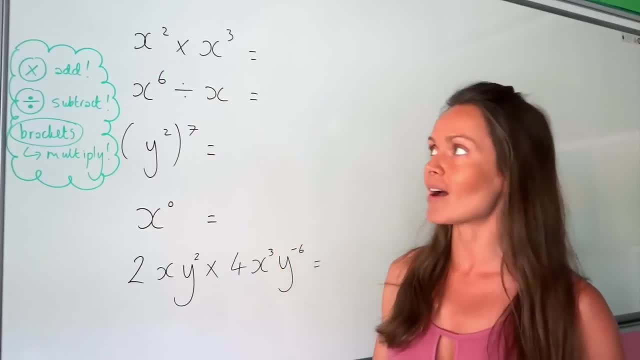 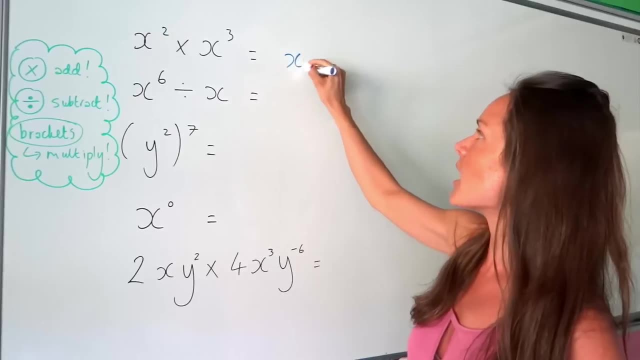 So I've got two letters that are the same. so the power rules apply, And because we're multiplying them together, we need to remember to add the powers. So in the first one I'm just doing 2 plus 3, which is 5.. Okay, on to the next one. 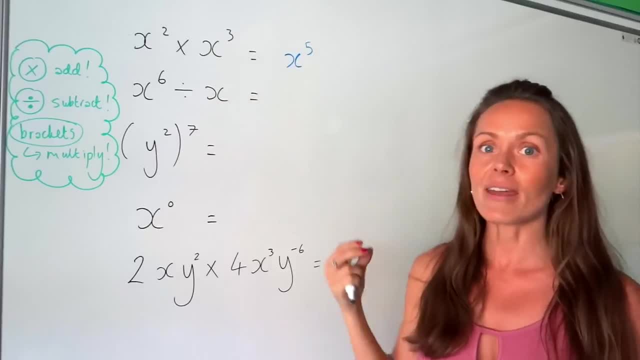 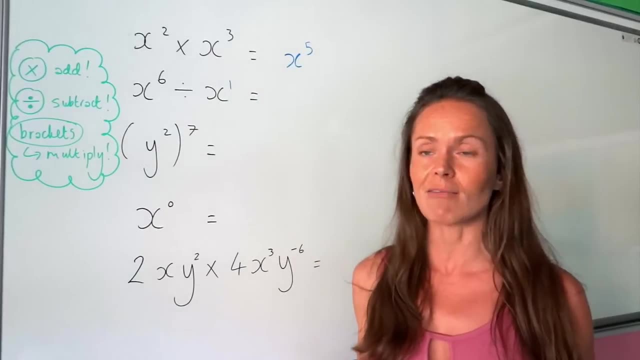 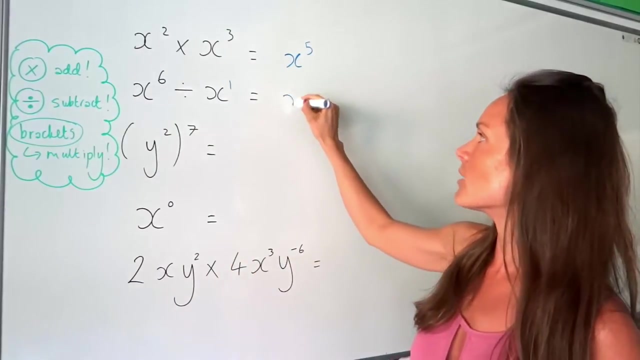 I just want to point out this x here There isn't a power on the x. It's up to you to remember. there's like an invisible 1 here that we don't normally write. So now we can subtract because, remember, when we're dividing you have to subtract the powers. So I write my x value down and 6. 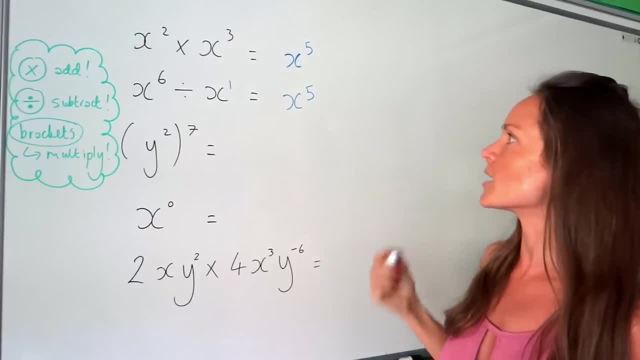 take away 1 is 5.. Okay, so we've got the same answer. Now on to the next one. This time we've got brackets. Whenever you see brackets, it means you must multiply the powers. So I'm just going to. 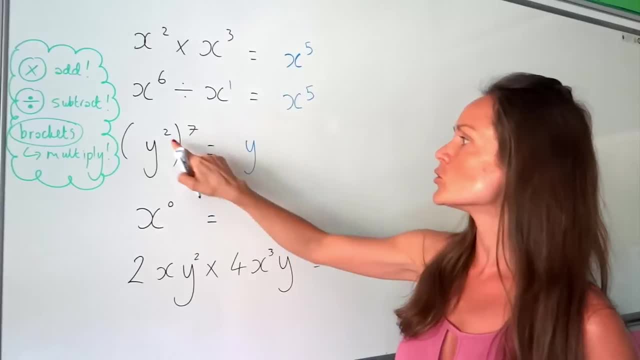 do this one. I just want to point out this x. here There isn't a power on the x, It's up to you to remember. multiply the powers together. So in this one, 2 multiplied by 7 is 14.. Now the fourth one is: 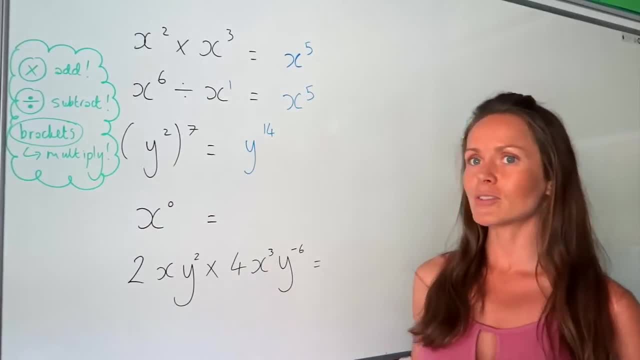 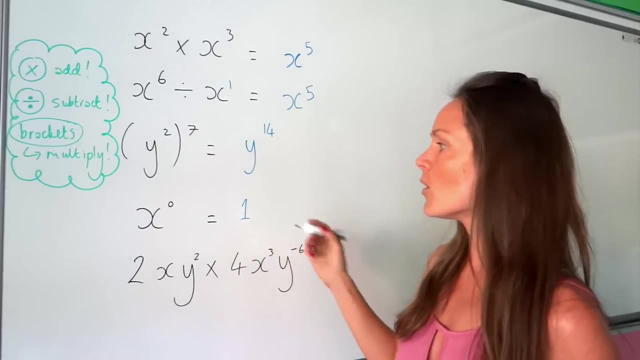 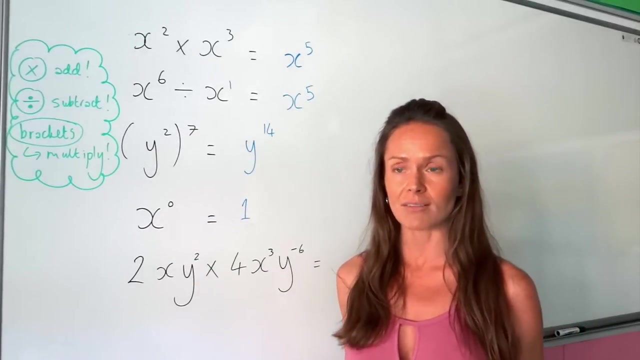 another rule, something else you need to remember: Whenever you see a letter or a number with the power of 0, the answer is just 1.. No matter what letter or what number you have, if you see the power of 0, it's always equal to the number 1.. Right on to the bottom one. So 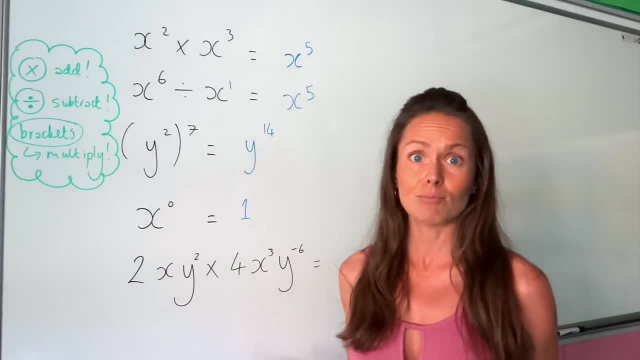 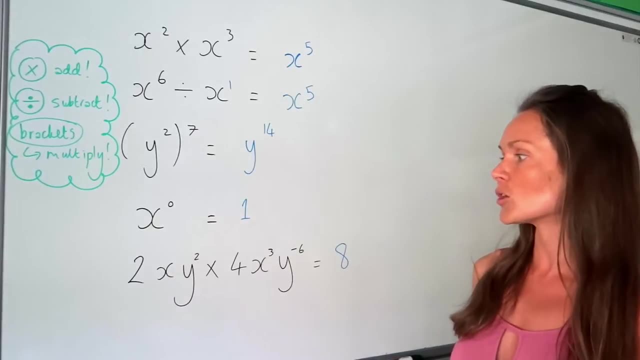 here I've got 2 times 4.. Well, we know how to multiply numbers. So 2 times 4 is just 8.. So you just multiply the numbers as normal. But now we're going to look at the powers, So remember that if 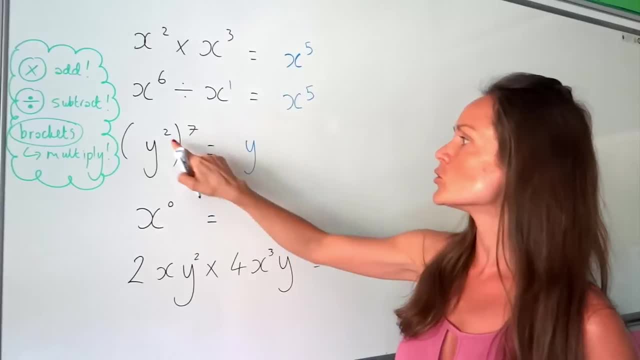 do this one. I just want to point out this x. here There isn't a power on the x, It's up to you to remember. multiply the powers together. So in this one, 2 multiplied by 7 is 14.. Now the fourth one is: 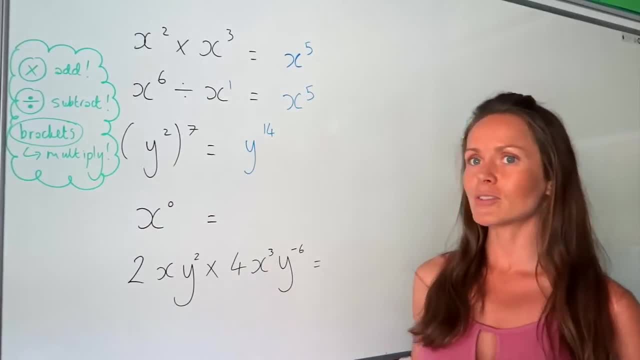 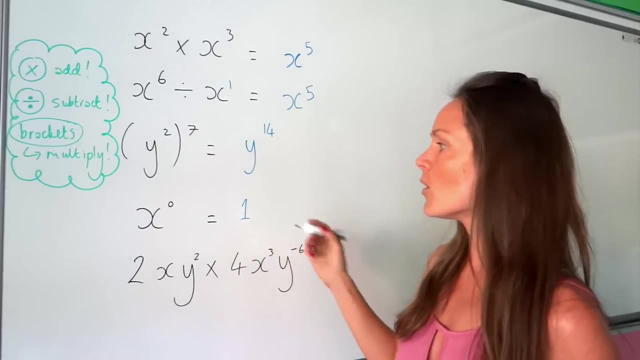 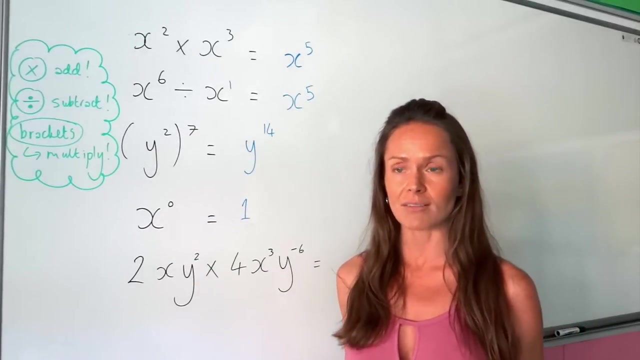 another rule, something else you need to remember: Whenever you see a letter or a number with the power of 0, the answer is just 1.. No matter what letter or what number you have, if you see the power of 0, it's always equal to the number 1.. Right on to the bottom one. So 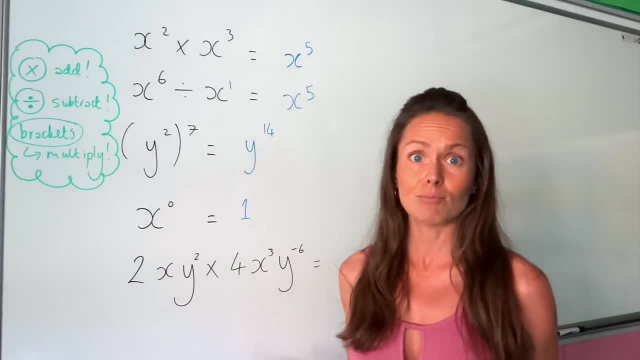 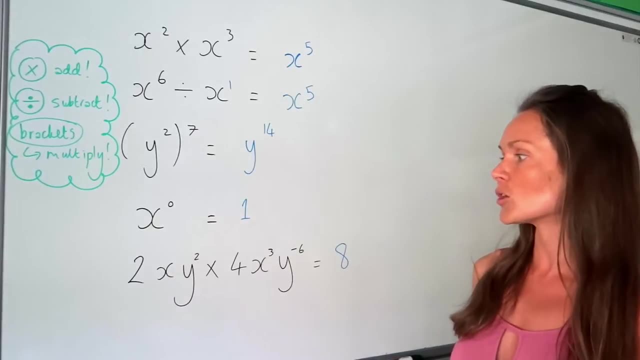 here I've got 2 times 4.. Well, we know how to multiply numbers. So 2 times 4 is just 8.. So you just multiply the numbers as normal. But now we're going to look at the powers, So remember that if 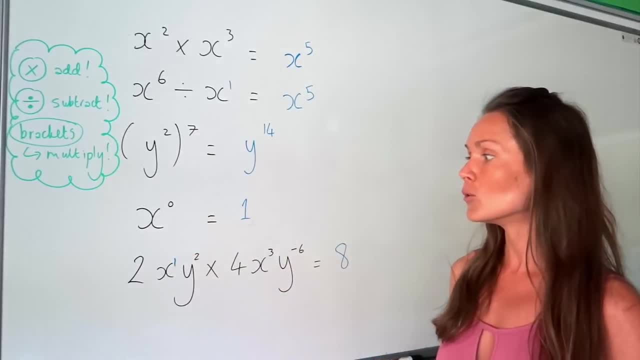 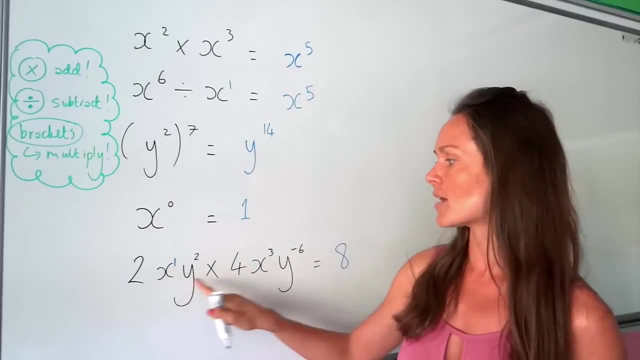 you don't see a power, there's like an invisible one here. And also remember the rules. the power rules only apply when the letter is the same. So first I'm going to look at the x values. So remember, for multiply you're adding the powers together. So I'm going to look at the x values. 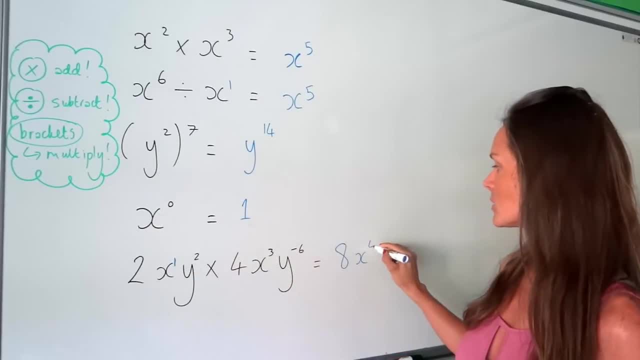 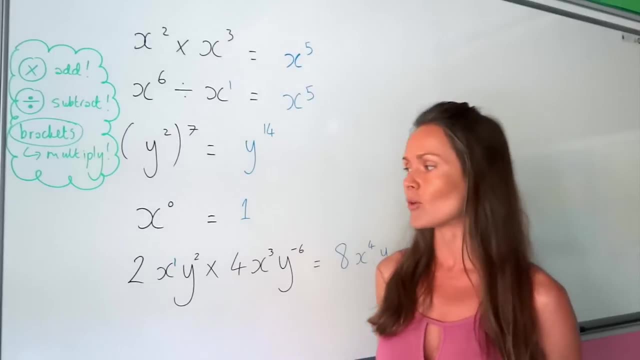 So for the x's we've got 1 plus 3, which is 4.. And now I'm going to look at the y values. So again it's multiplied. So we're adding the powers together on the y letters. So 2 plus negative 6 is 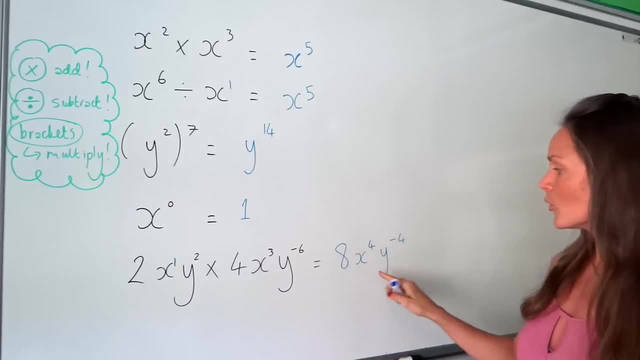 negative 4.. And we can't do anything else with this. We can't times these letters together. OK, because the power rules only work if the letter is the same and these letters are different. OK, now I'm going to make them a bit harder. 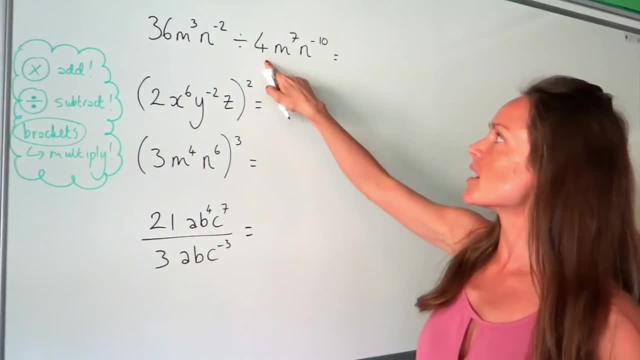 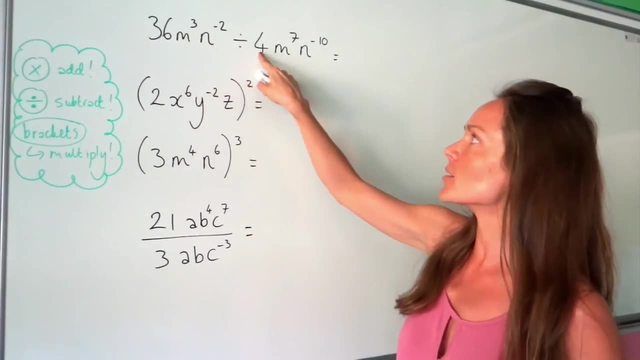 OK, so in this top one up here I'm dividing. Remember, if you just see normal numbers, you just divide them as normal. So 36 divided by 4 is just equal to the number 9.. And now I'm going. 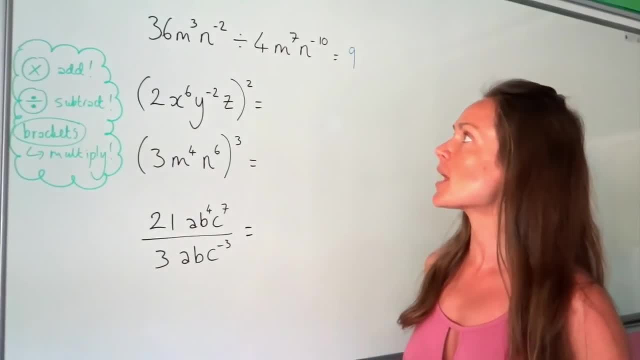 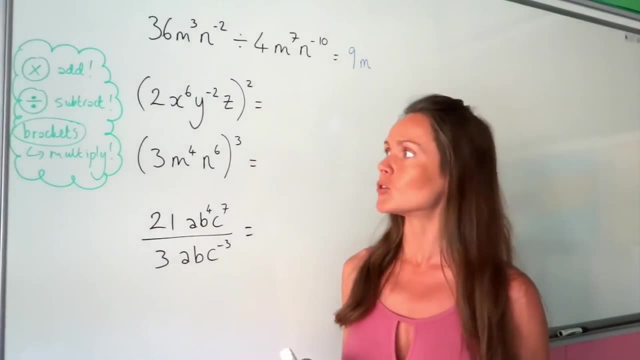 to look at the letters individually to work out what happens to the powers. So first I'm going to look at the n values, So I'm going to write down n And remember, for divide you have to subtract the powers. So for the m we've got 3. And we're going to divide by 4.. And now I'm going to 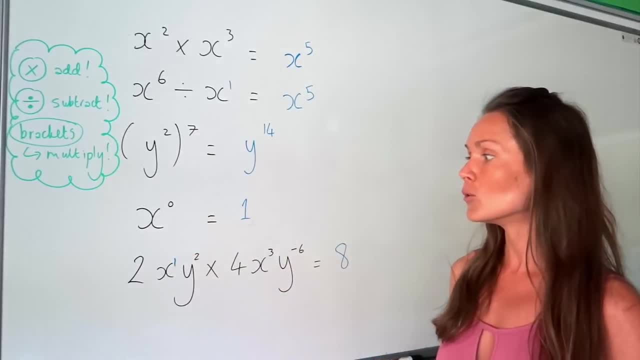 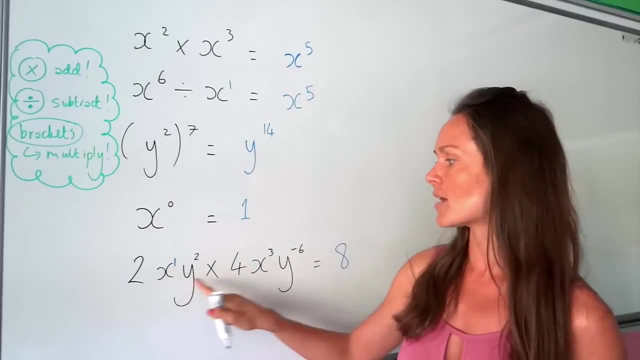 you don't see a power, there's like an invisible one here. And also remember the rules. the power rules only apply when the letter is the same. So first I'm going to look at the x values. So remember, for multiply you're adding the powers together. So I'm going to look at the x values. 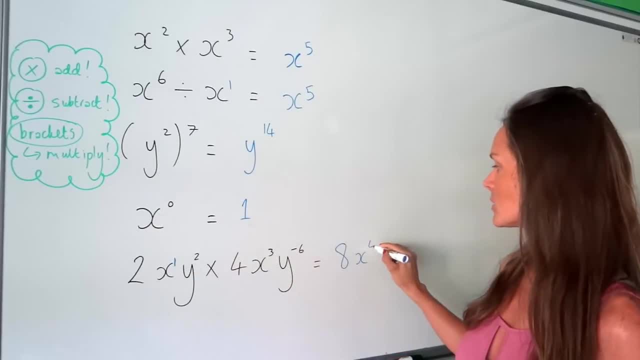 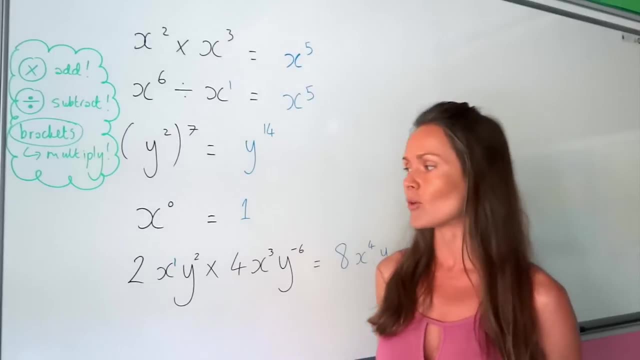 So for the x's we've got 1 plus 3, which is 4.. And now I'm going to look at the y values. So again it's multiplied. So we're adding the powers together on the y letters. So 2 plus negative 6 is 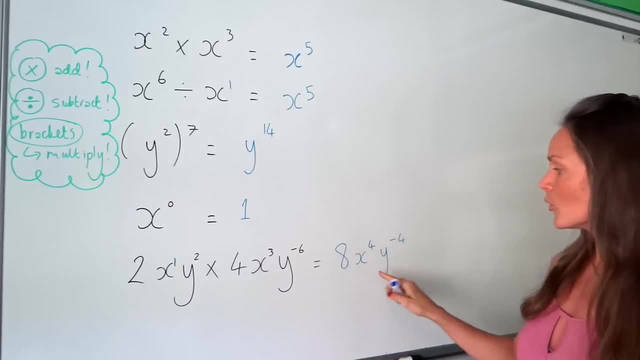 negative 4.. And we can't do anything else with this. We can't times these letters together. OK, because the power rules only work if the letter is the same and these letters are different. OK, now I'm going to make them a bit harder. 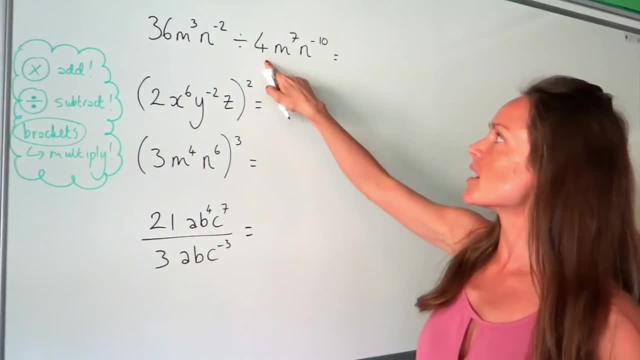 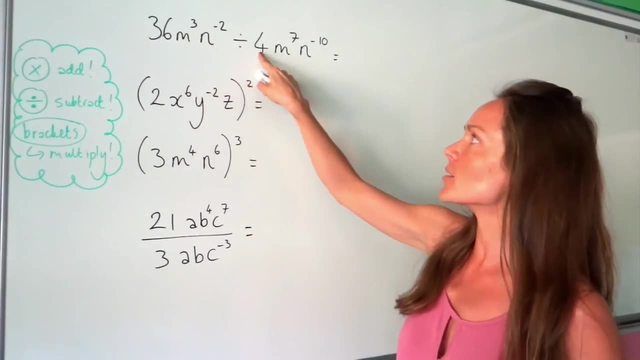 OK, so in this top one up here I'm dividing. Remember, if you just see normal numbers, you just divide them as normal. So 36 divided by 4 is just equal to the number 9.. And now I'm going. 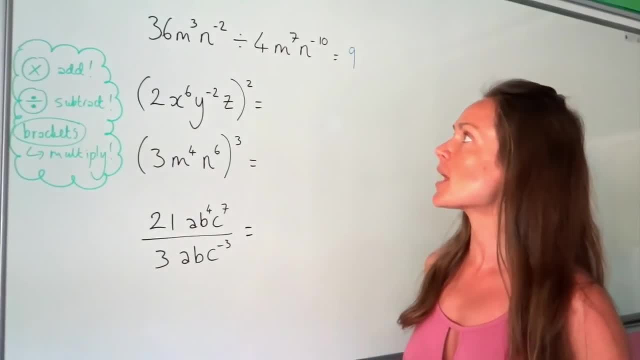 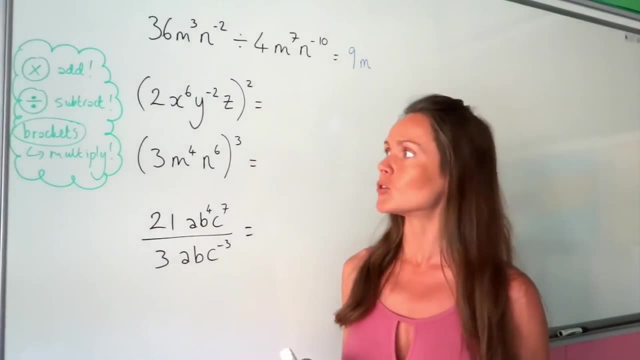 to look at the letters individually to work out what happens to the powers. So first I'm going to look at the n values, So I'm going to write down n And remember, for divide you have to subtract the powers. So for the m we've got 3. And we're going to divide by 4.. And now I'm going to 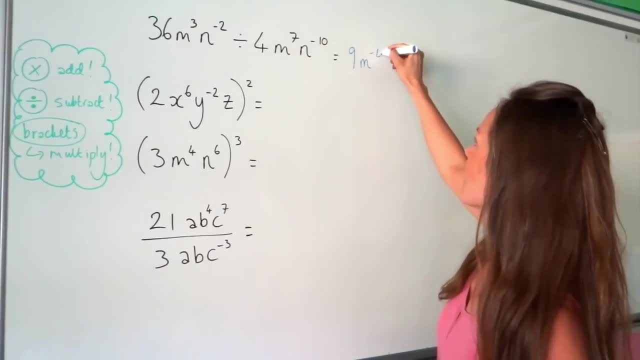 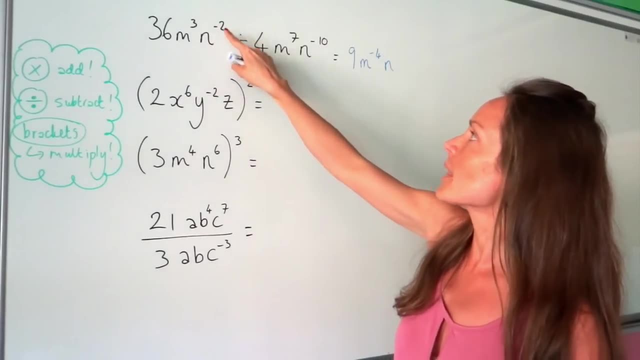 take away 7, which is negative 4.. And now I'm going to look at the n values. So again I'm subtracting the powers, So I've got minus 2, take away negative 10.. So be careful there, because 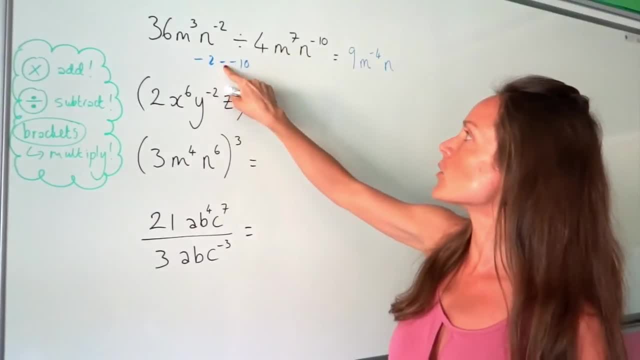 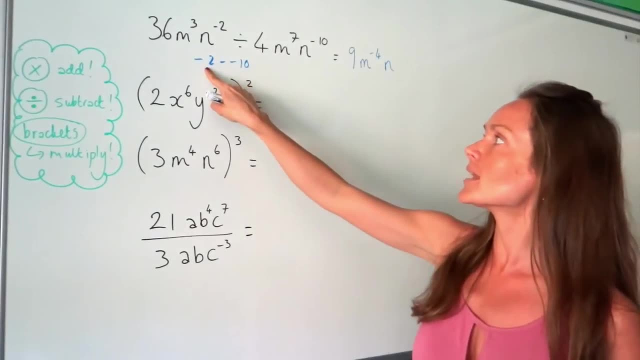 you've got a double minus, You're doing minus 2, take away And then this happens to be negative. Remember, when you see two negatives together like this, they turn into a plus. So negative 2 plus 10 is equal to 8.. So that gives me the power. So I'm going to subtract the powers. And now I'm going to. 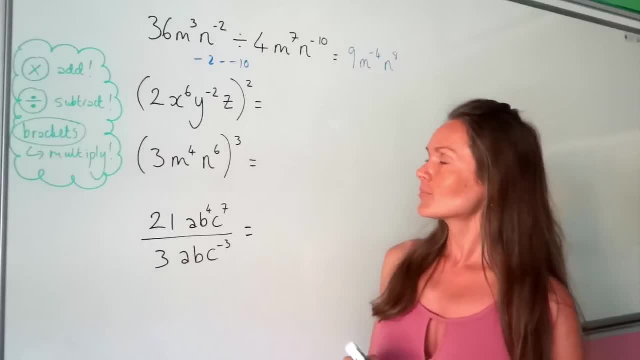 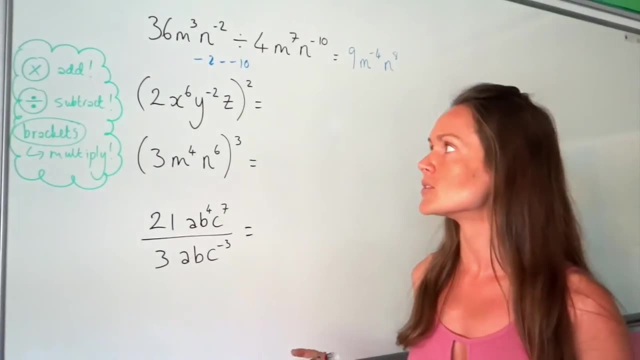 take away the power on the n, So that one's done. Now this one here. lots of people make mistakes on this one because they see the brackets And they think, great, I'm going to multiply the powers. But then they forget about this number here. Remember this: squared affects everything. 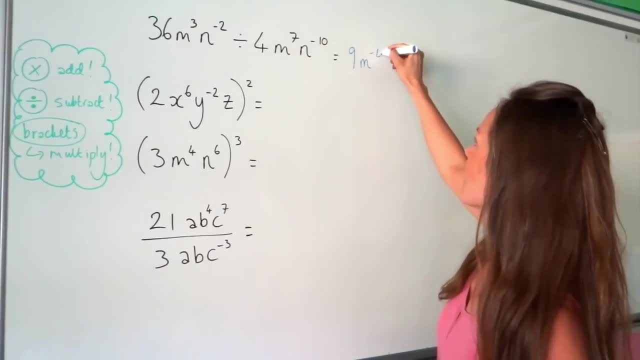 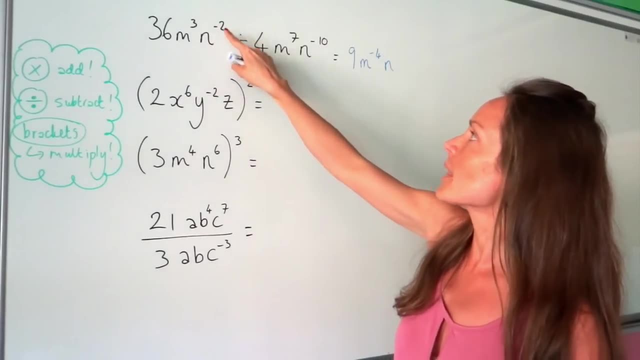 take away 7, which is negative 4.. And now I'm going to look at the n values. So again I'm subtracting the powers, So I've got minus 2, take away negative 10.. So be careful there, because 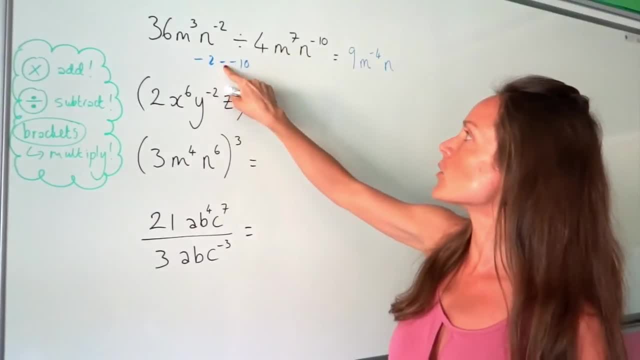 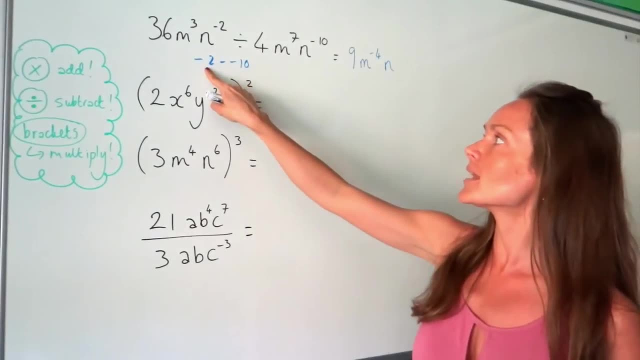 you've got a double minus, You're doing minus 2, take away And then this happens to be negative. Remember, when you see two negatives together like this, they turn into a plus. So negative 2 plus 10 is equal to 8.. So that gives me the power. So I'm going to subtract the powers. And now I'm going to. 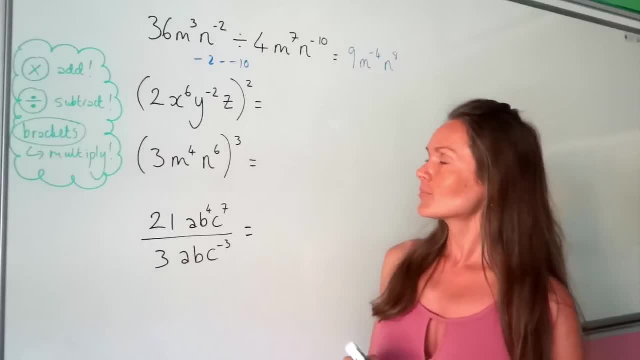 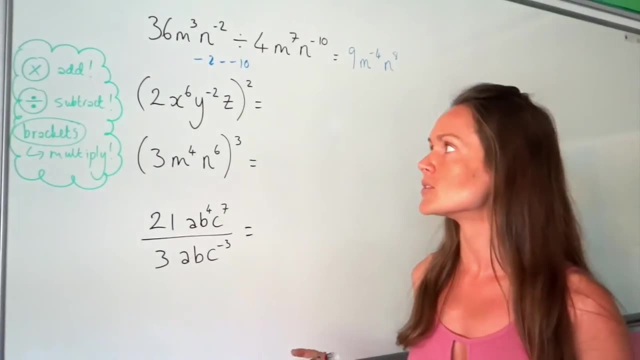 take away the power on the n, So that one's done. Now this one here. lots of people make mistakes on this one because they see the brackets And they think, great, I'm going to multiply the powers. But then they forget about this number here. Remember this: squared affects everything. 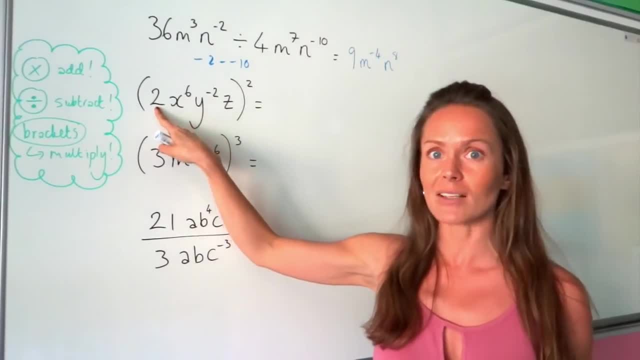 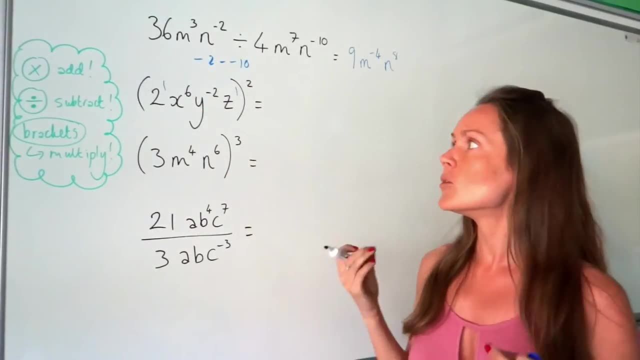 inside the brackets. So you have to square this number 2 as well. So this 2, don't forget this- has like an invisible power of 1 that we wouldn't normally write, But you need to remember that it's still there. 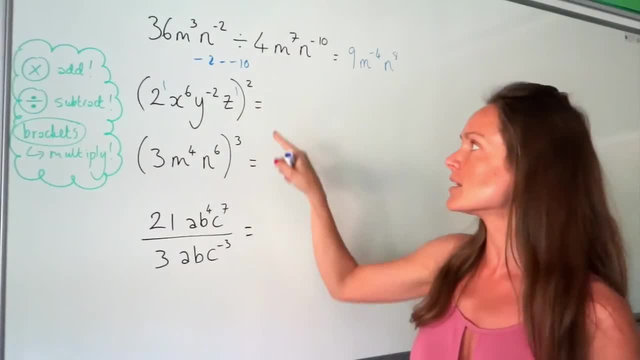 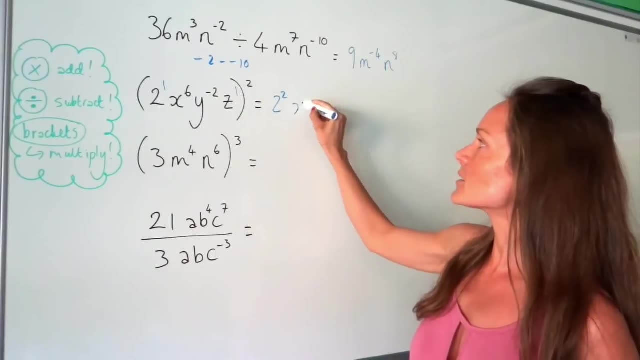 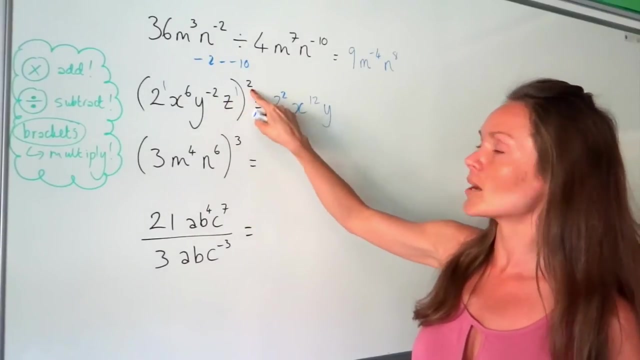 So you have to multiply every single power inside the brackets by 2.. So that would give me 1 times 2, is just 2.. For the x value, you've got 6 times 2, which is 12.. For the y value, we've got minus 2. 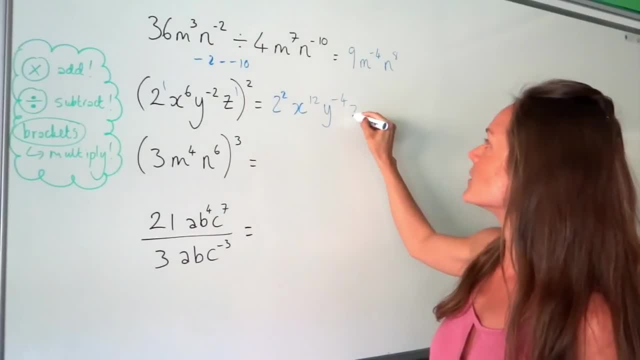 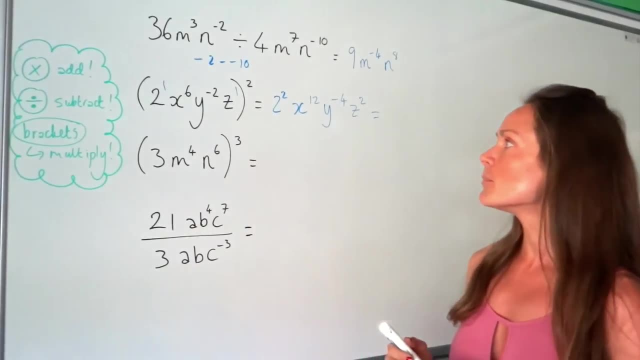 times 2,, which is minus 4.. And lastly, for the z, 1 times 2,, which is 2.. Now, that's correct, But we can simplify this a little bit, Because 2 squared. we can work that out. 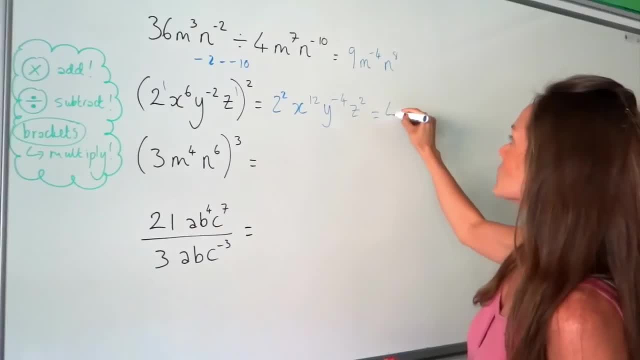 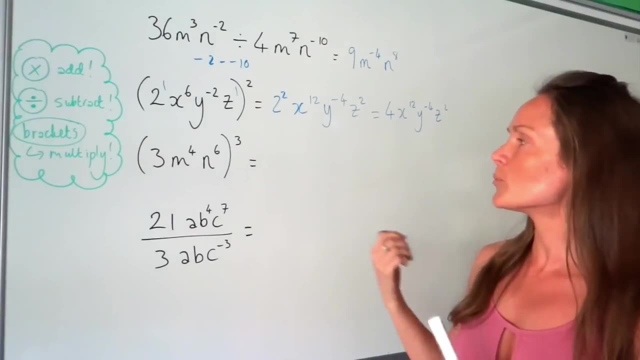 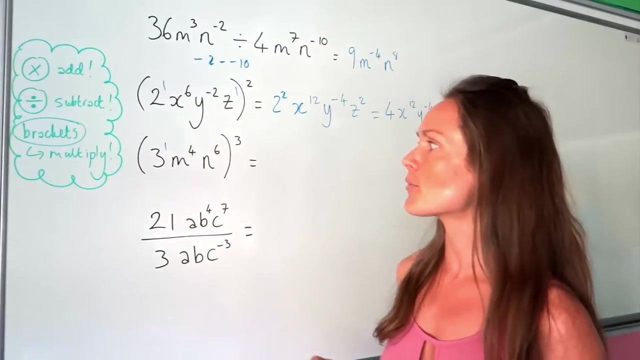 2 squared is 2 times 2,, which is 4.. So I'm just going to write my final version like that. OK? So, just like in the previous example, remember this power affects everything inside the brackets, So even that number 3 at the beginning. So remember to multiply all the. 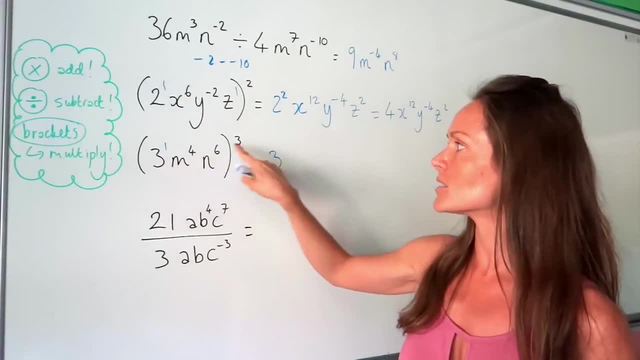 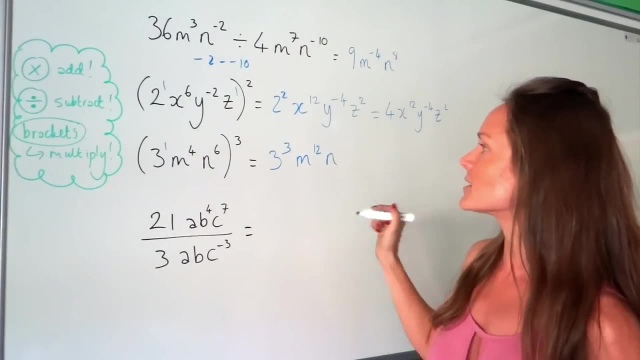 powers here by 3.. So this one 1 times 3 is just 3.. For the n value we've got 4 times 3., Which is 12.. And lastly n 6 times 3,, which is 18.. And again, just evaluate that here. 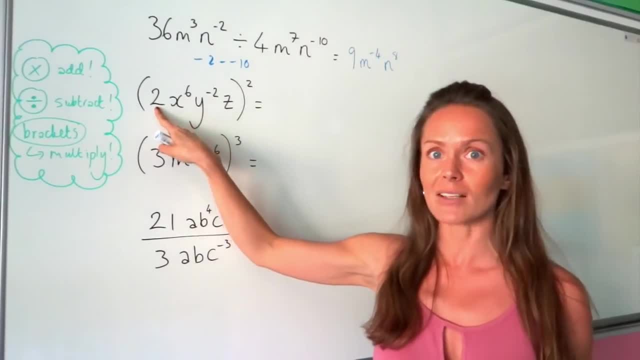 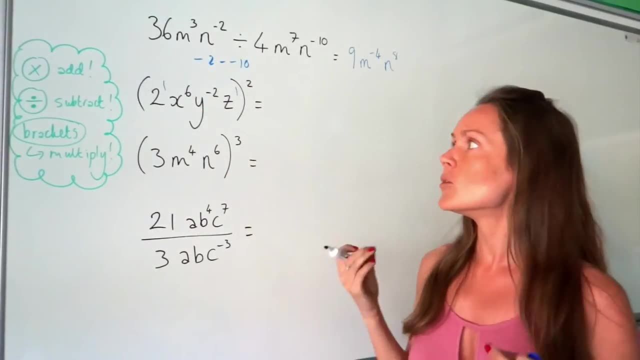 inside the brackets. So you have to square this number 2 as well. So this 2, don't forget this- has like an invisible power of 1 that we wouldn't normally write, But you need to remember that it's still there. 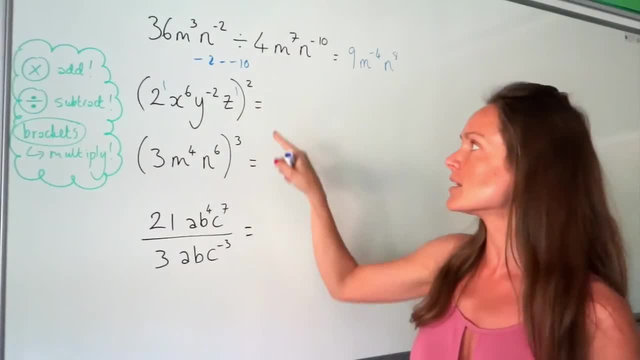 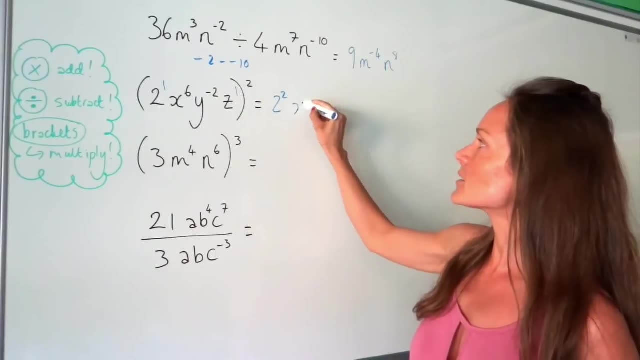 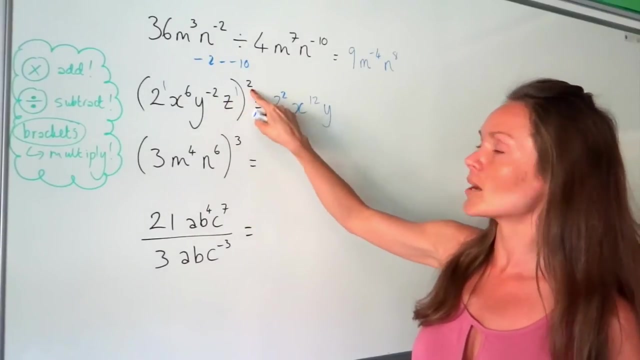 So you have to multiply every single power inside the brackets by 2.. So that would give me 1 times 2, is just 2.. For the x value, you've got 6 times 2, which is 12.. For the y value, we've got minus 2. 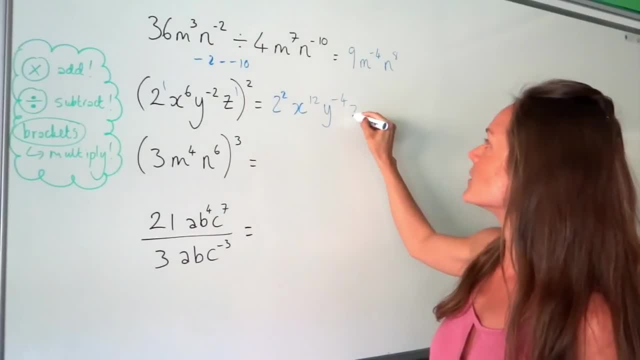 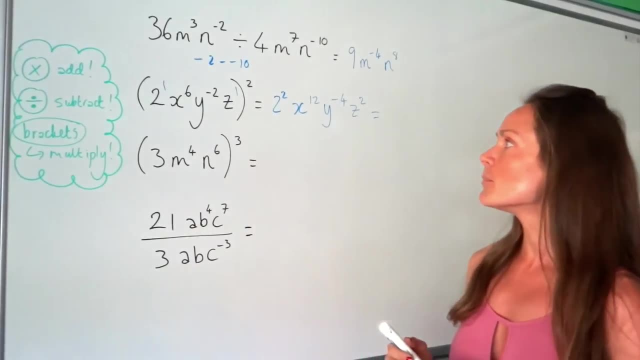 times 2,, which is minus 4.. And lastly, for the z, 1 times 2,, which is 2.. Now, that's correct, But we can simplify this a little bit, Because 2 squared. we can work that out. 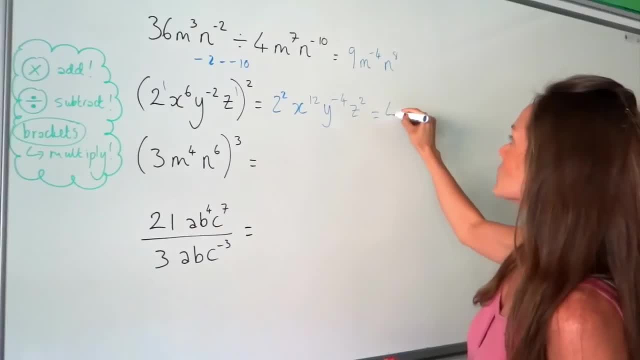 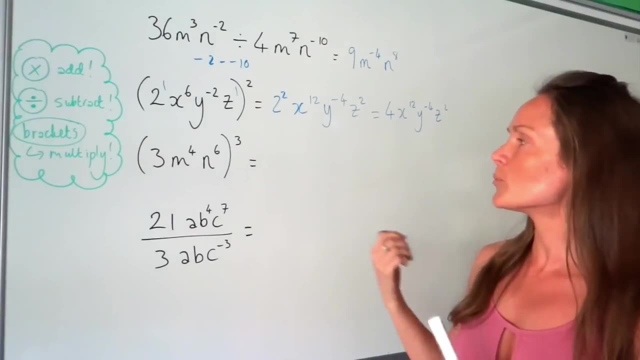 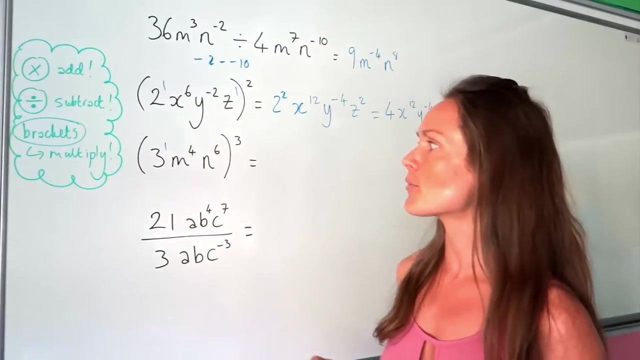 2 squared is 2 times 2,, which is 4.. So I'm just going to write my final version like that. OK? So, just like in the previous example, remember this power affects everything inside the brackets, So even that number 3 at the beginning. So remember to multiply all the. 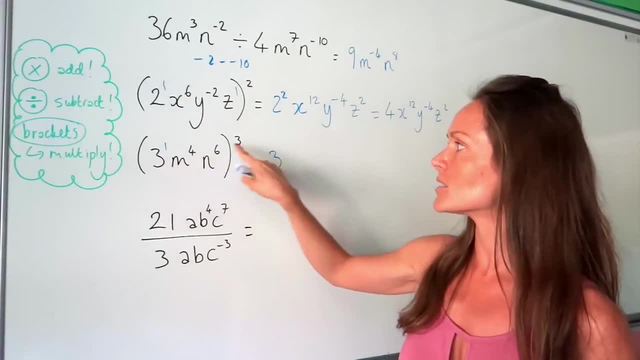 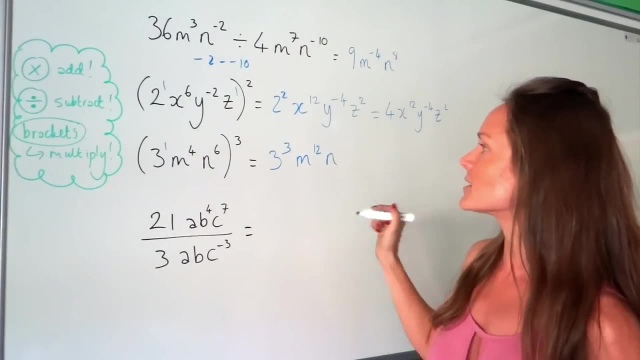 powers here by 3.. So this one 1 times 3 is just 3.. For the n value we've got 4 times 3., Which is 12.. And lastly n 6 times 3,, which is 18.. And again, just evaluate that here. 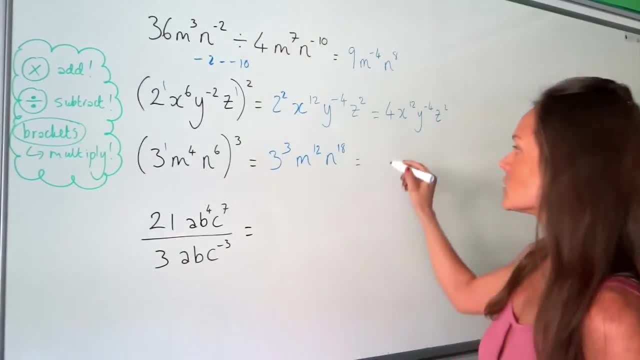 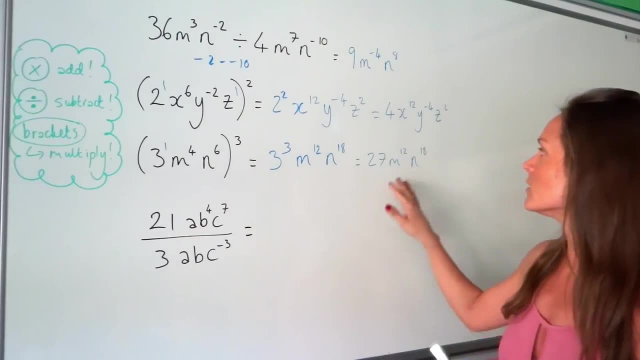 3 cubed. 3 cubed is 3 times 3 times 3, which is 27.. And everything else stays the same. Remember: you can't do anything else with these letters here, because they're different letters. So the rules, the power rules, don't apply when you have different letters. So 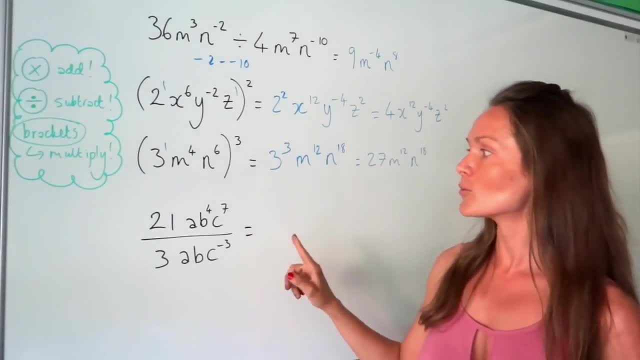 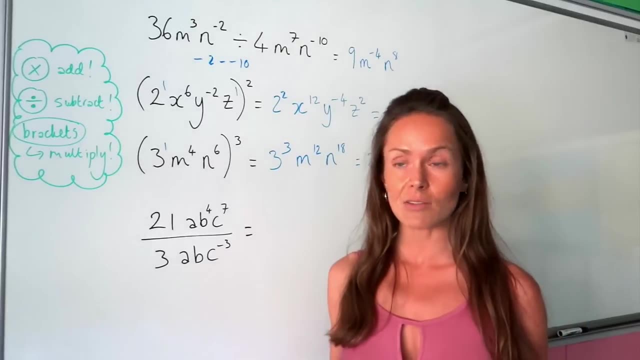 that's finished. Now on to this one here. So this one is actually just like the one at the top. here It's divide. Remember, when you see a fraction, that just means divide. So we're doing the numerator divided by the denominator. 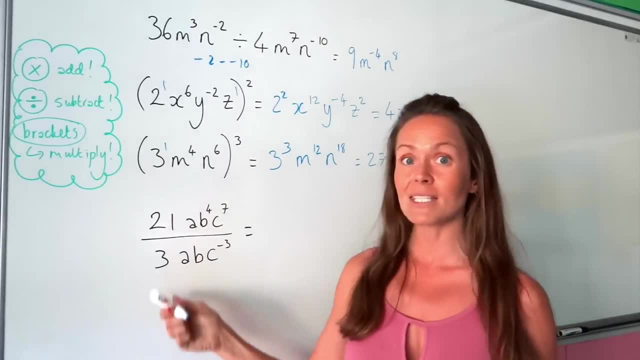 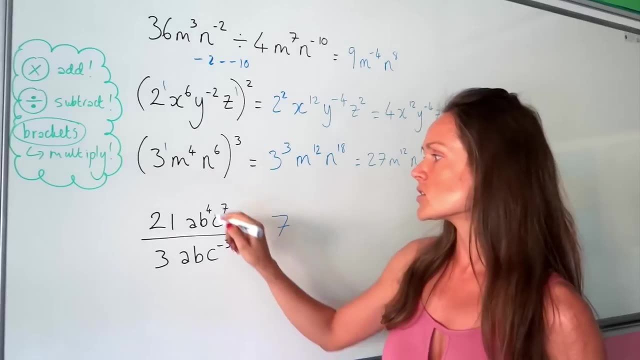 So we're going to look at the numbers. first of all, We've got 21 divided by 3, which we can work out, It's just 7.. And now I'm going to look at the letter a. So remember there's. 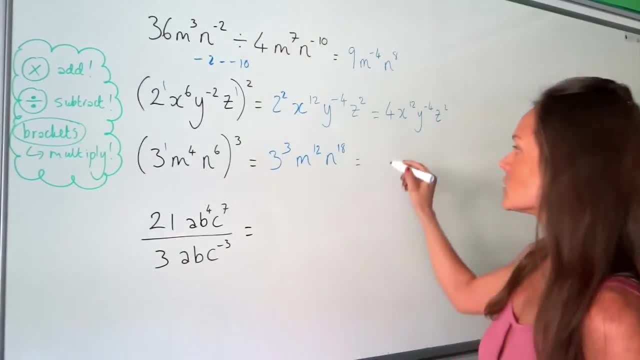 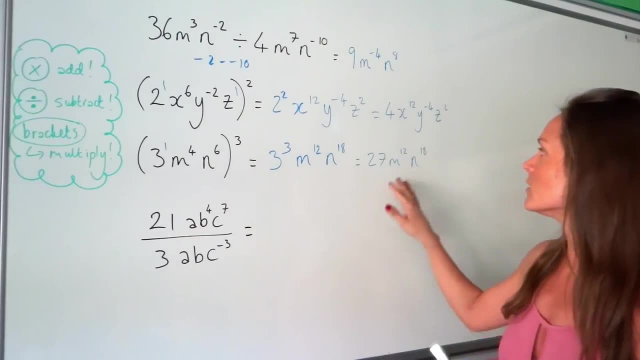 3 cubed. 3 cubed is 3 times 3 times 3, which is 27.. And everything else stays the same. Remember: you can't do anything else with these letters here, because they're different letters. So the rules, the power rules, don't apply when you have different letters. So 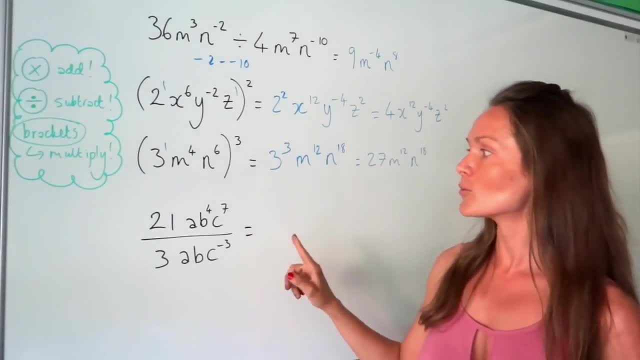 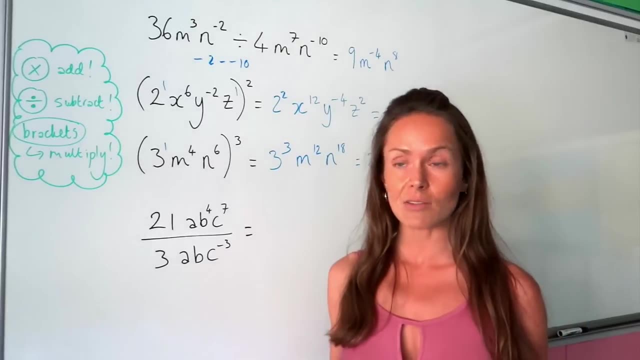 that's finished. Now on to this one here. So this one is actually just like the one at the top. here It's divide. Remember, when you see a fraction, that just means divide. So we're doing the numerator divided by the denominator. 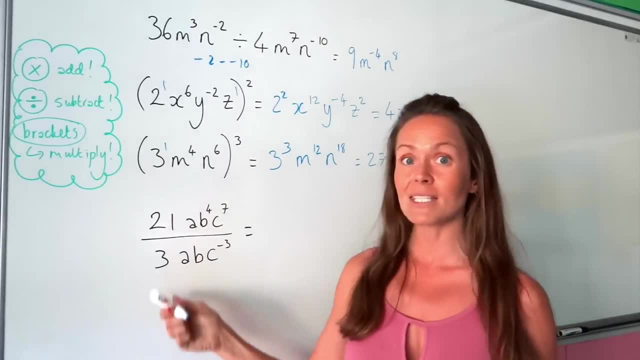 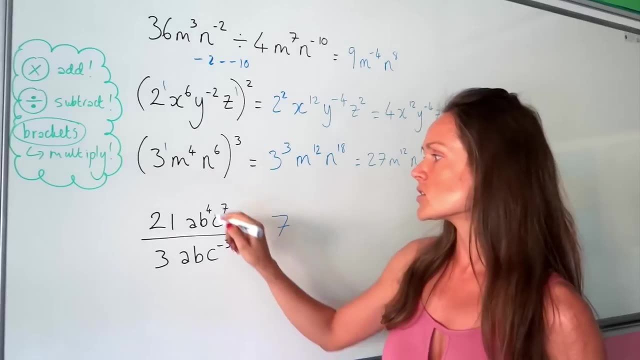 So we're going to look at the numbers. first of all, We've got 21 divided by 3, which we can work out, It's just 7.. And now I'm going to look at the letter a. So remember there's. 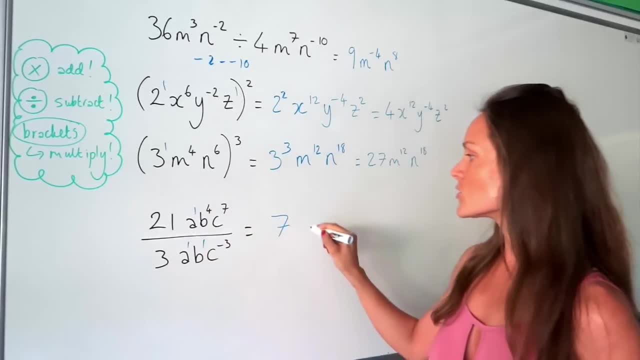 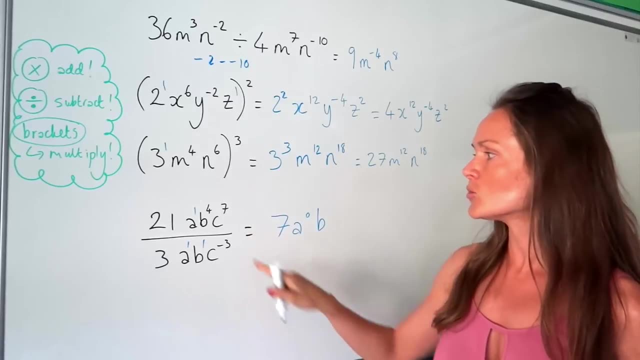 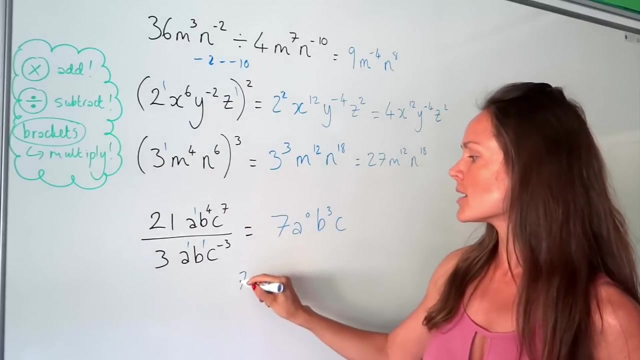 like an invisible 1 on these letters that don't have powers. So for the a, well, 1, take away 1 is just 0.. For the b values, we've got 4, take away 1, which is 3.. And for the c, we've got 7, take. 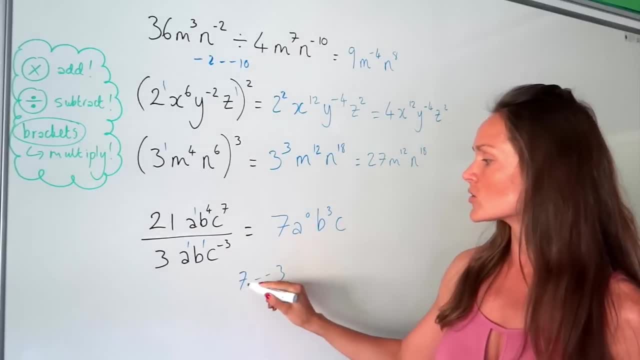 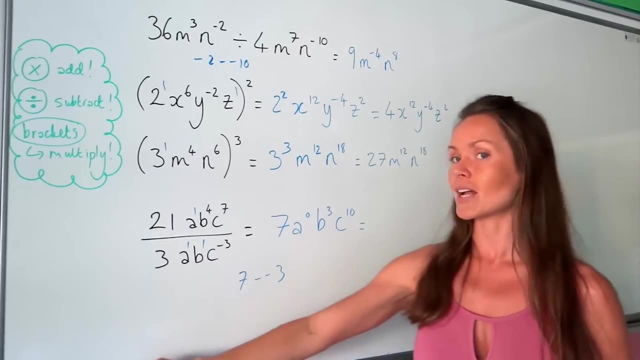 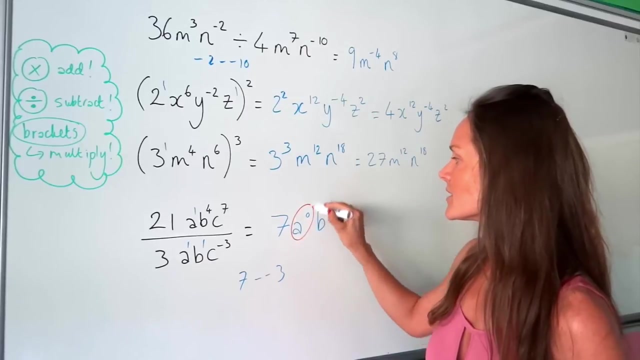 away. negative 3.. Watch out for the double minus. So 7 plus 3,, which is 10.. But I can do something else with this one. Remember earlier I told you that any letter or any number that has a power of 0 is equal to the number 1.. Well, I can see here I've got a. 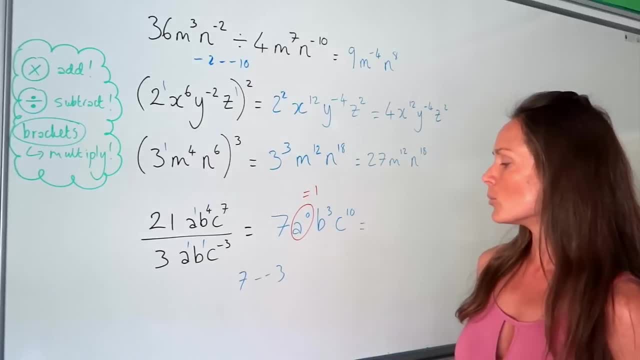 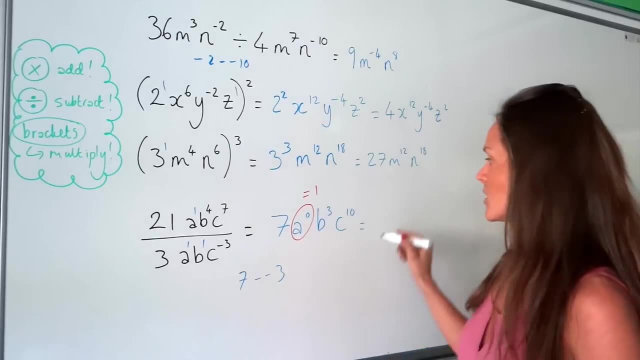 to the power of 0.. Which is equal to 1.. Well, these are all being multiplied together, So if this is 1, 7 times 1 is just 7.. So I can just tidy that up a little bit and write it like that, So that: 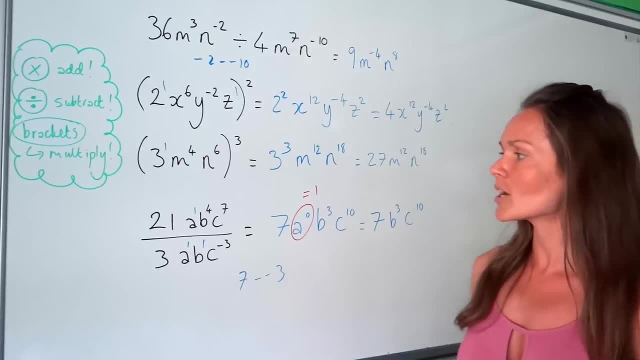 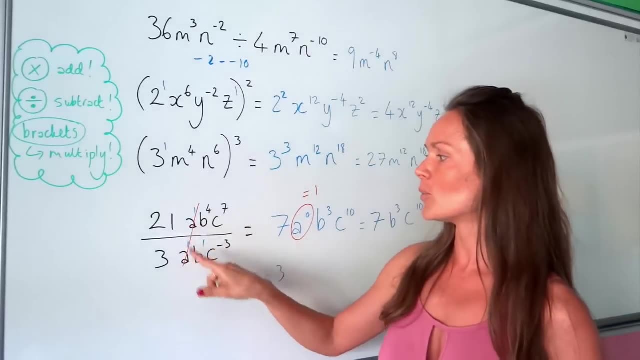 makes sense because if I look over here when I'm dividing, we could have actually just crossed those out straight away, Because whenever you divide something by itself- so a to the 1, divided by a to the 1, well, they just cancel each other out. So if I look over here, I 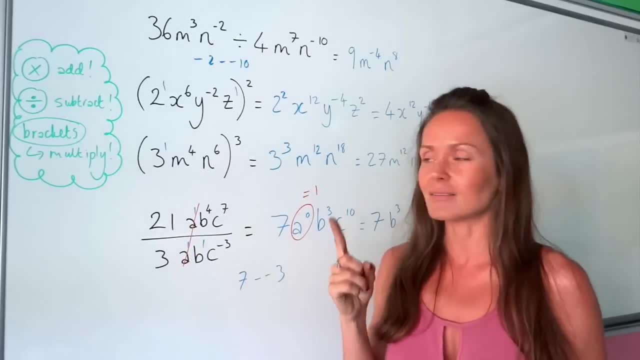 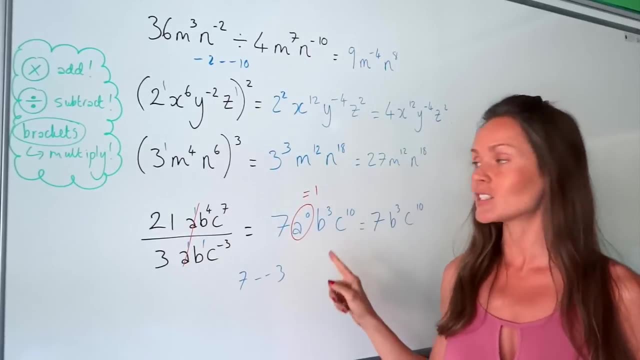 can see that everything is justCómo. if you look over here, you could have crossed out each other, because how many a1's in a1? Just 1.. OK, So you could have crossed them out there. Or if you forget to do that and you see this over here, just remember anything to the power. 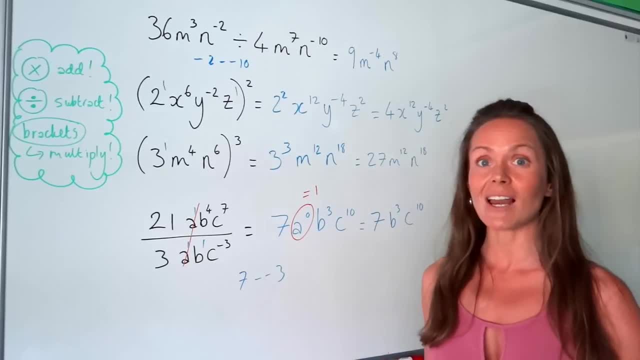 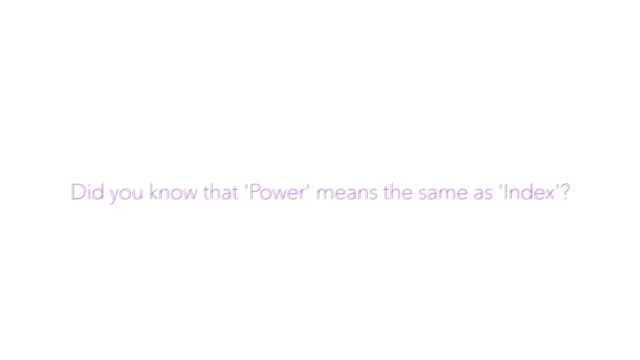 of 0 is equal to 1.. OK, I've got one more challenge question to finish. All right, So in this last example, it's not really that it's more difficult, It's just a long question with lots of working out. So what I'm doing here is: I'm going to add: 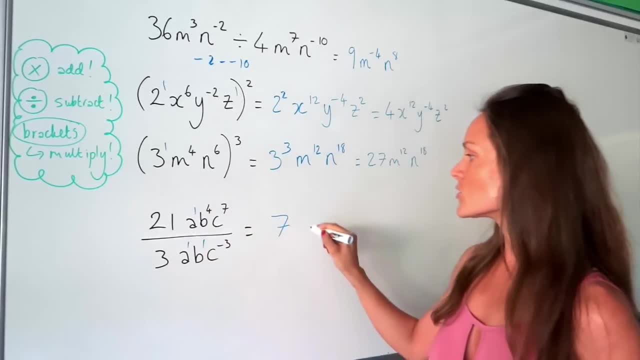 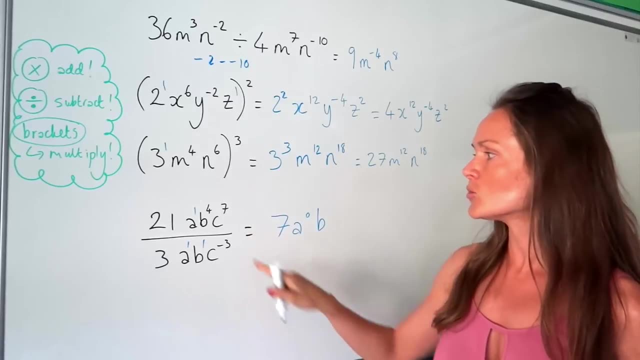 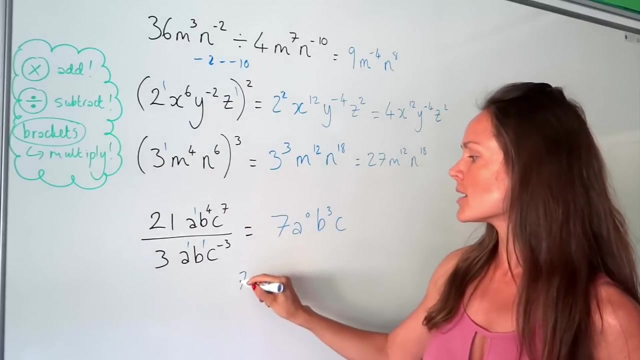 like an invisible 1 on these letters that don't have powers. So for the a, well, 1, take away 1 is just 0.. For the b values, we've got 4, take away 1, which is 3.. And for the c, we've got 7, take. 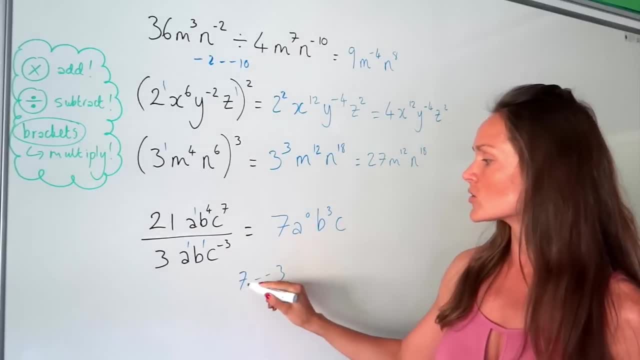 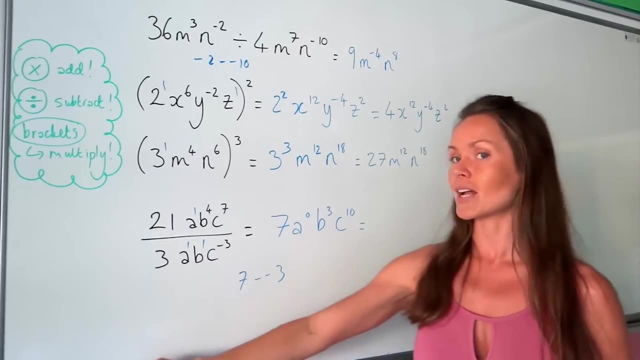 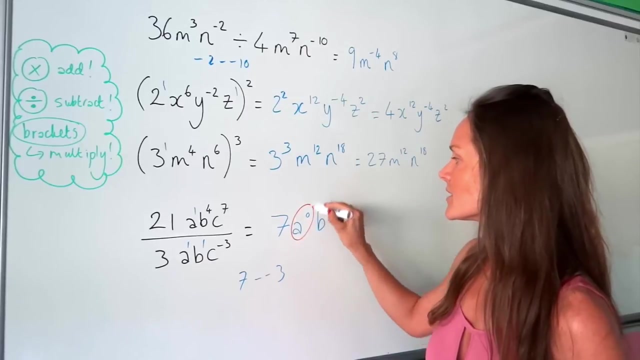 away. negative 3.. Watch out for the double minus. So 7 plus 3,, which is 10.. But I can do something else with this one. Remember earlier I told you that any letter or any number that has a power of 0 is equal to the number 1.. Well, I can see here I've got a. 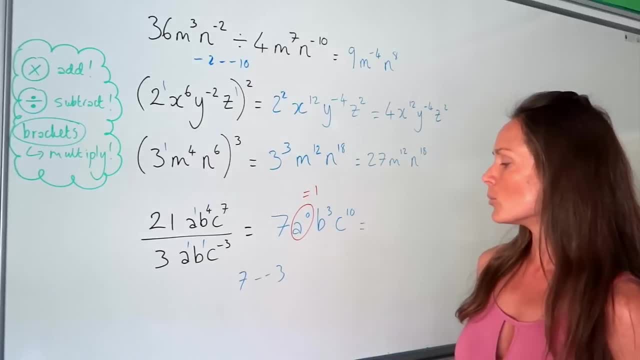 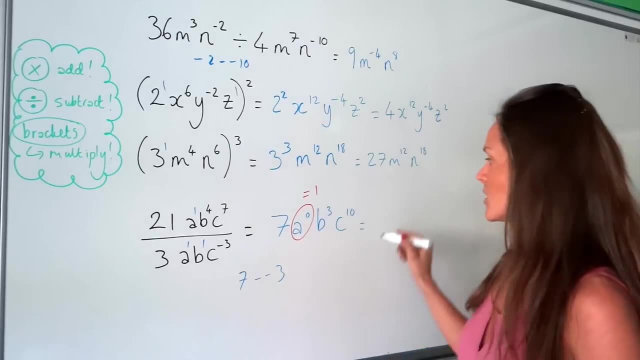 to the power of 0.. Which is equal to 1.. Well, these are all being multiplied together, So if this is 1, 7 times 1 is just 7.. So I can just tidy that up a little bit and write it like that, So that: 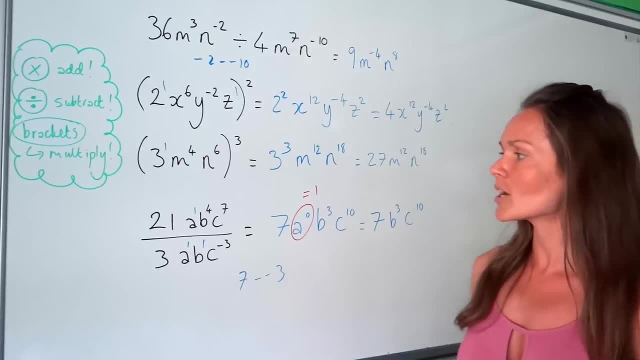 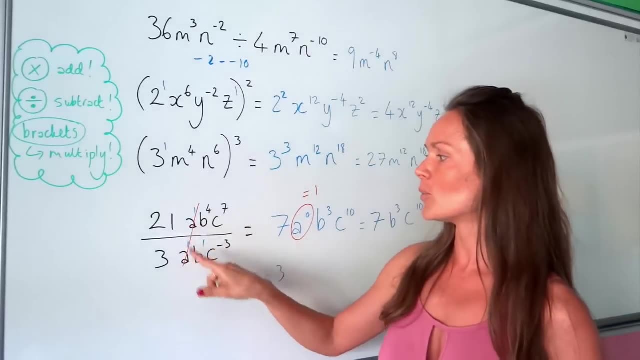 makes sense because if I look over here when I'm dividing, we could have actually just crossed those out straight away, Because whenever you divide something by itself- so a to the 1, divided by a to the 1, well, they just cancel each other out. So if I look over here, I 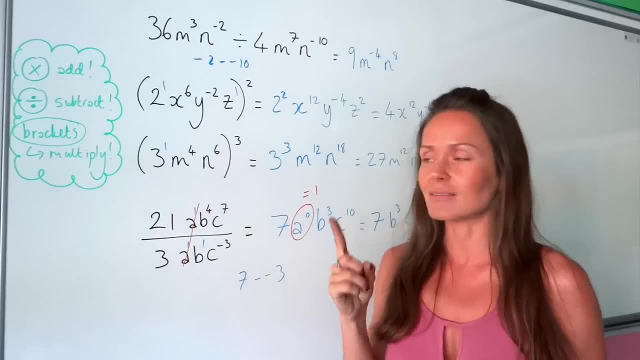 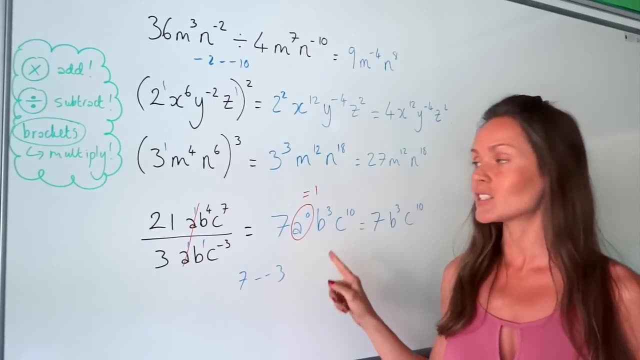 see, I'm just crossing each other out, Because how many a1s and a1? Just one. OK, so you could have crossed them out there. Or if you forget to do that and you see this over here, just to remember, anything to the power of 0 is equal to 1.. OK, I've got one more challenge. 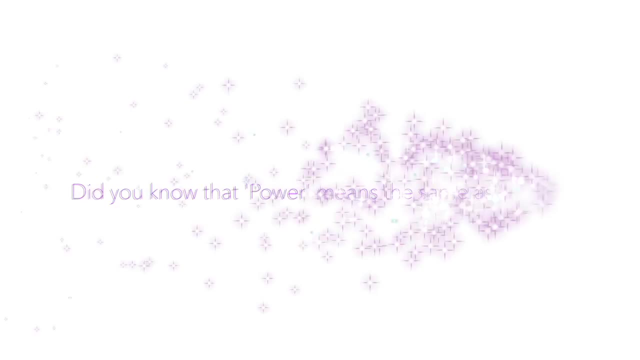 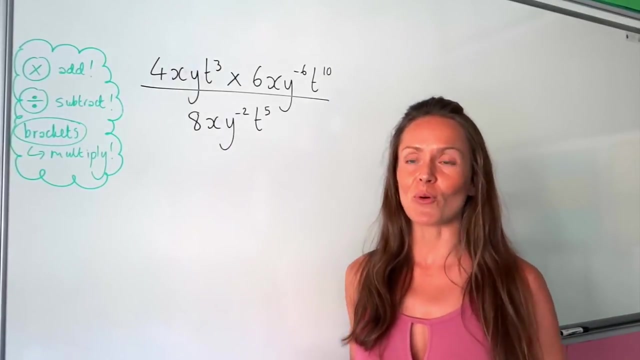 question to finish, All right. So in this last example it's not really that it's more difficult, It's just a long question with lots of working out. So let's say you're a realist And we know you're a rich world, But you're a realist. So let's say you've got a little bit of a. 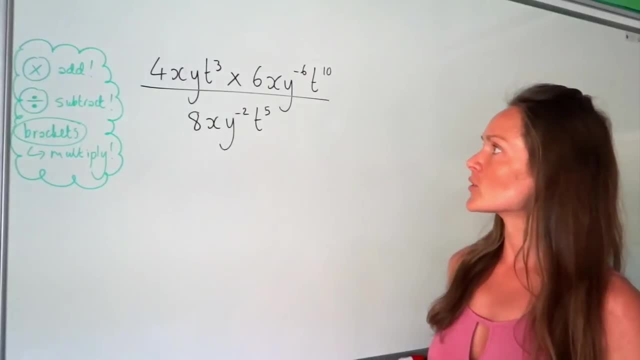 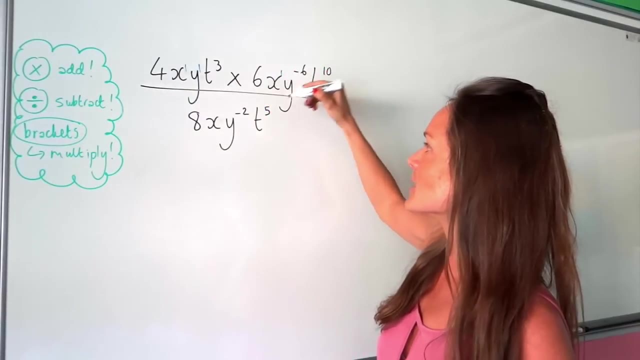 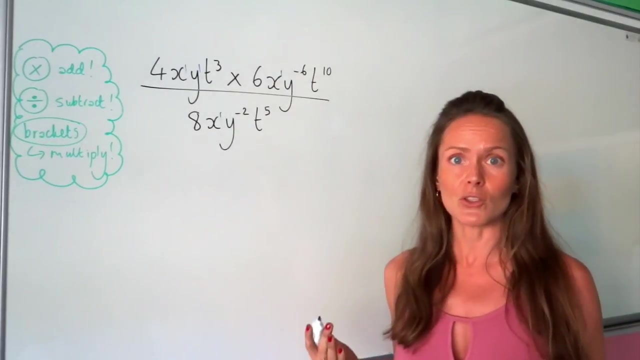 I'm not showing you any new rules, so in this first one, just before I get started, so I don't forget to do it later on- I'm going to just add the powers of one to all of those letters that don't have powers. okay, and now I'm going to get started, so I'm going to work out what happens to the. a two. I'm going to add a two, I'm going to add a 2. And I'm going to add a 3. And I'm going to add a 5.. So I'm going to add a 5.. So I'm going to add a 4.. And then I'm going 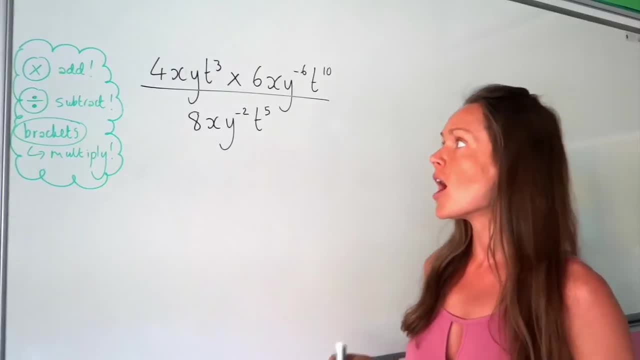 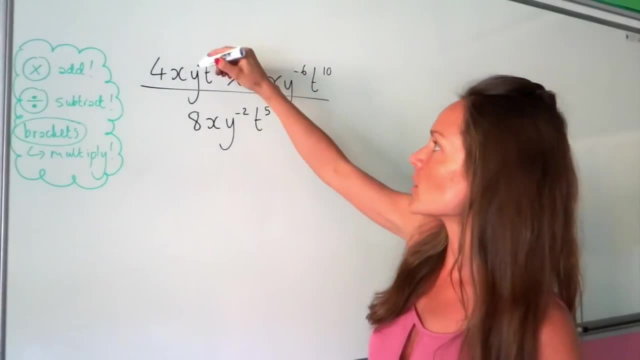 it's more difficult. It's just a long question with lots of working out. I'm not showing you any new rules, So in this first one, just before I get started- so I don't forget to do it later on- I'm going to just add the powers of one to all of those letters that. 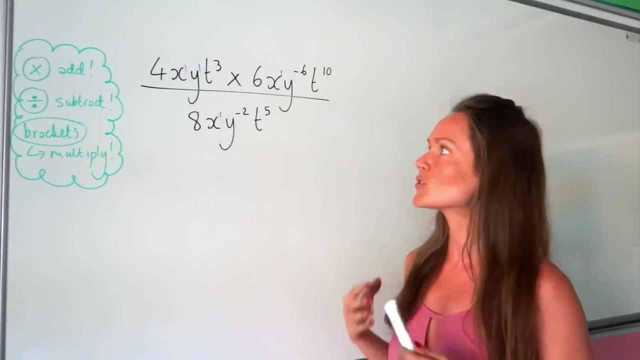 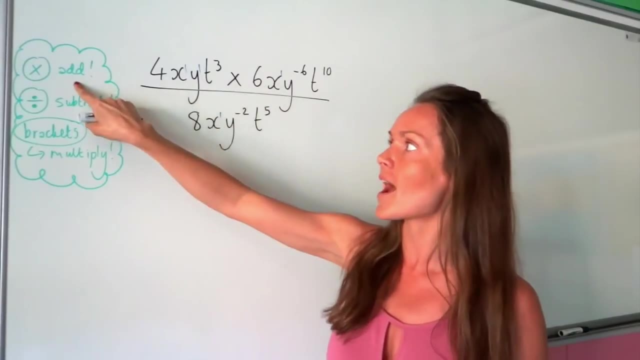 don't have powers. Okay, and now I'm going to get started. So I'm going to work out what happens to the numerator. to start with, Remember, when you're multiplying, you must add all the powers together. So, firstly, the numbers four and six. well, I'm just multiplying those. 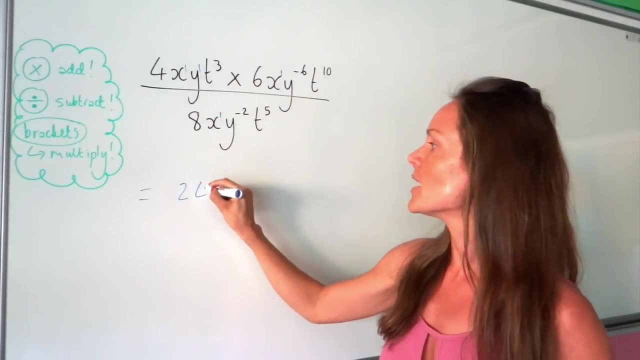 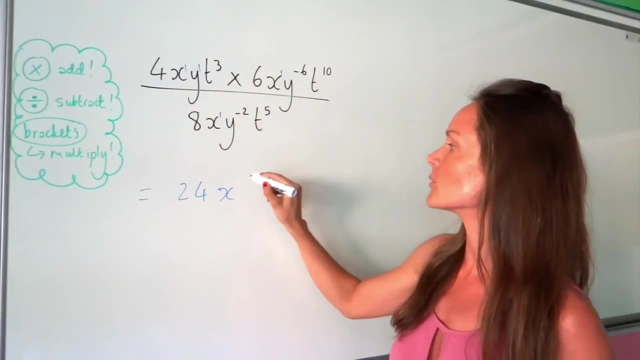 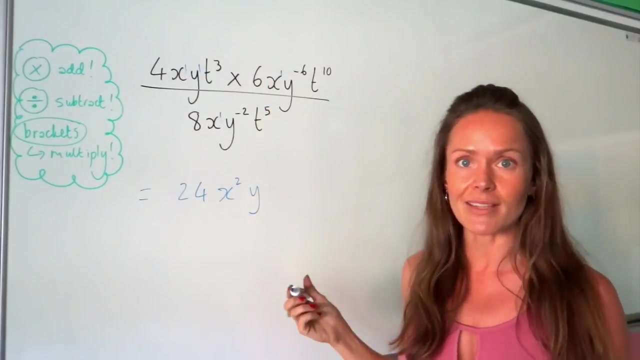 numbers as normal. So four times six is 24.. Now I'm going to look at the x values and I'm going to add their powers together. So for the x values, you've got one plus one, which is two. Okay, now for the y values, we've got one plus negative six, which is. 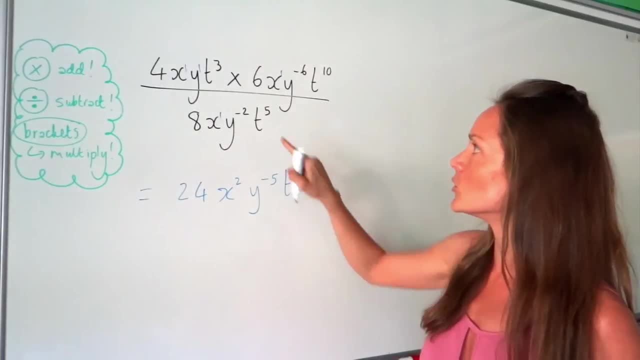 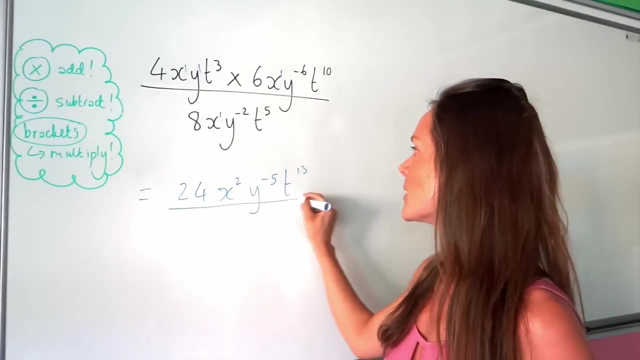 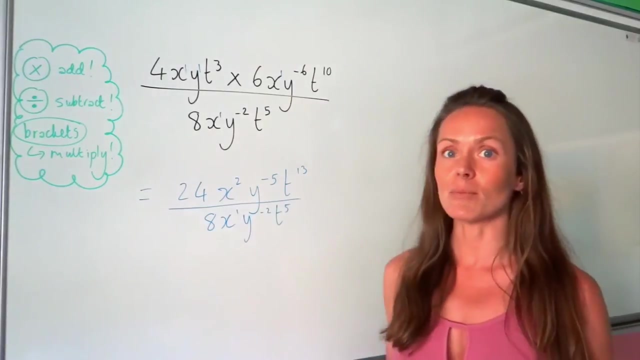 negative five, And finally the t values, and we've got three plus 10, which is five. Okay, so I've added all the powers together. Now this denominator is still there. it hasn't changed just yet. And remember, when you see a fraction like this, it means we're dividing. 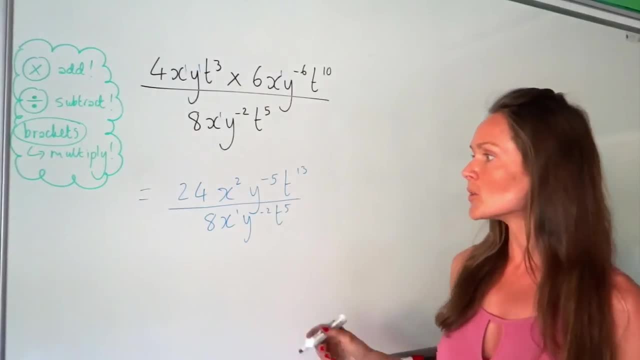 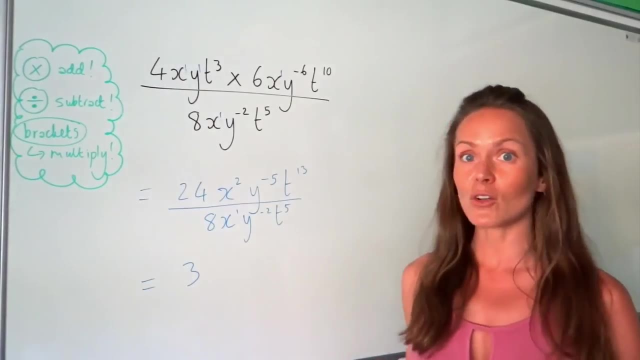 so we're subtracting the powers. So the numbers just as before. you just divide those as normal. So 24 divided by eight is just three. Now I'm going to look at the x values. So I'm subtracting, I'm doing two. take away one, which is just one. 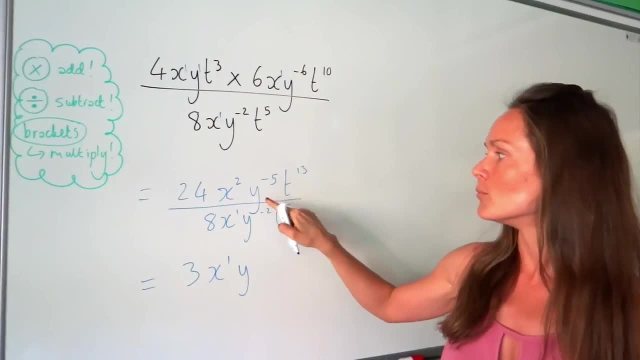 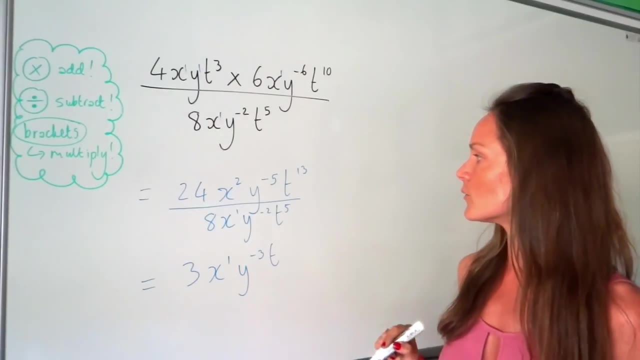 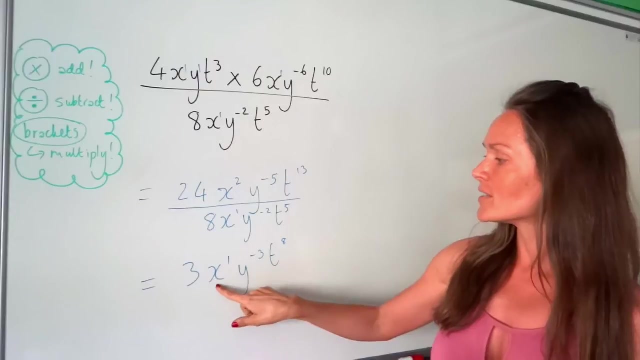 Now for the y values. I've got minus five minus minus two, which is the same as minus five plus two, which is minus three. And lastly for the t values, 13, take away five, which is just eight. Okay, so for this x value, here I did write to the power of one, But remember. 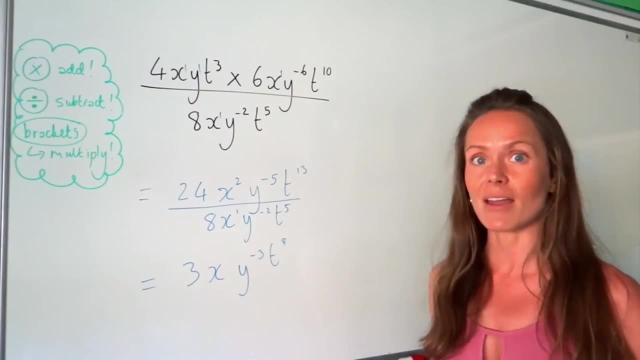 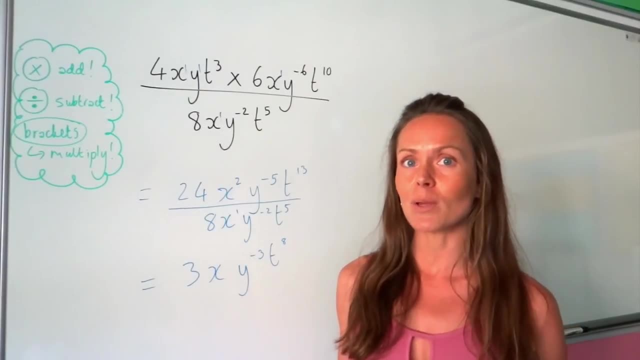 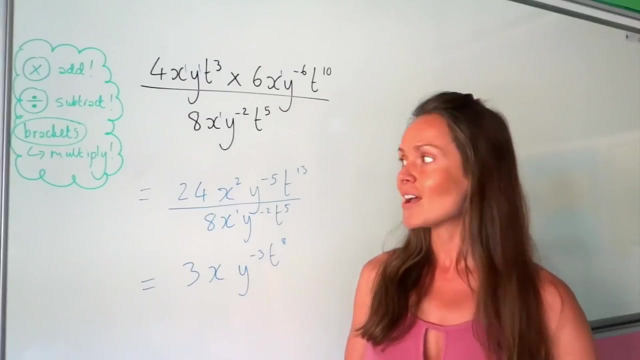 you don't have to write that, okay, you can just leave it like that. So they're the basic rules of indices, the power rules. I will have another video with other rules, harder questions, but that's more for the extended syllabus, So it may not be in your end exam. So, anyway, that's all from me for today and goodbye.